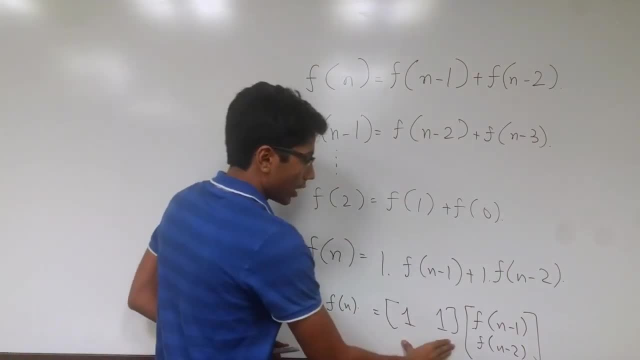 way that we look at Fibonacci numbers. Okay, f of n is a multiplication of two matrices, one of which is f of n minus 1 plus f of n minus 2.. One of which has one 1, and the other one has terms of the Fibonacci sequence from: 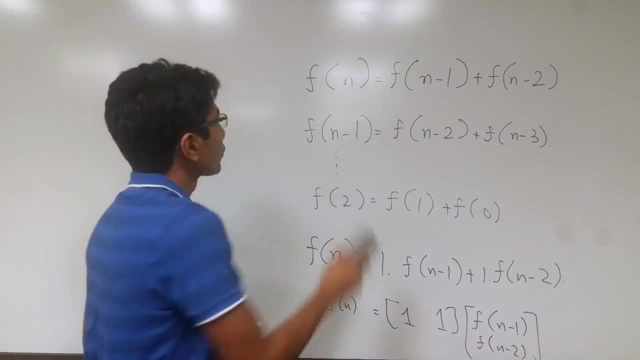 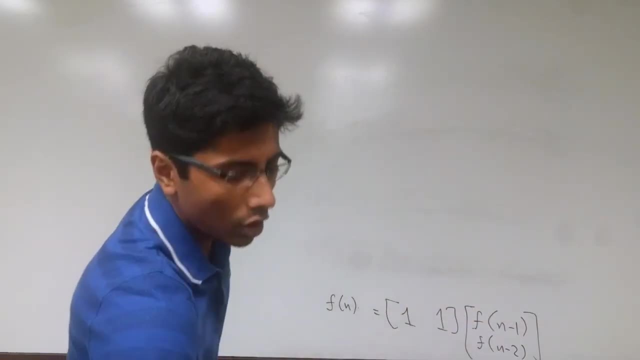 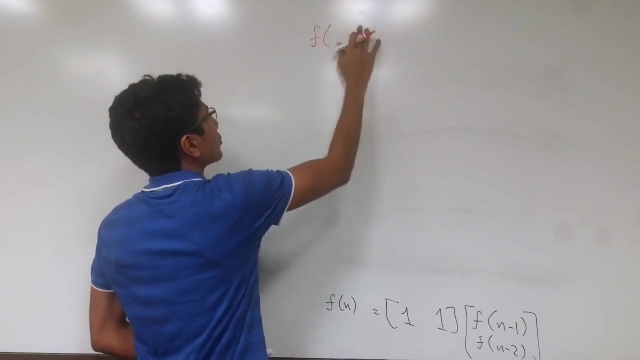 previously. So let's take some examples. Let's take the first three terms of the Fibonacci sequence. That's f of n minus- no, it's not n anymore, so that's f of 2 is equal to well, that is equal to 1 into 1,. 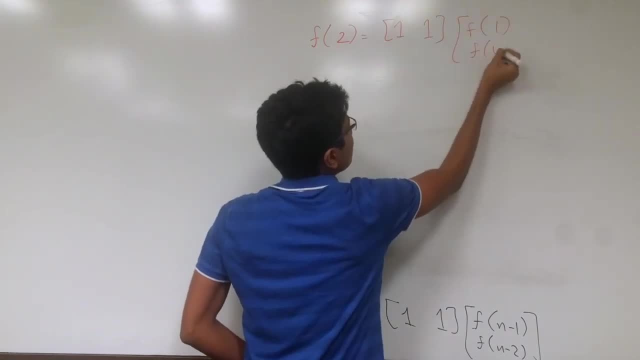 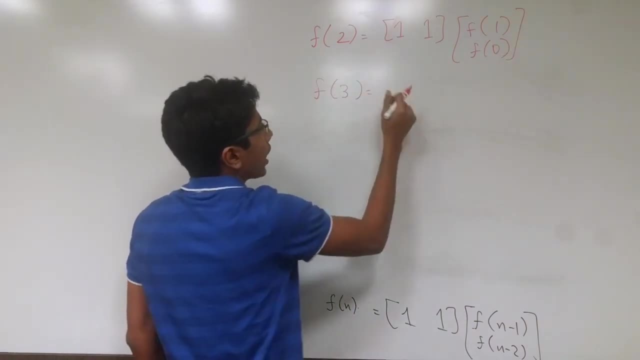 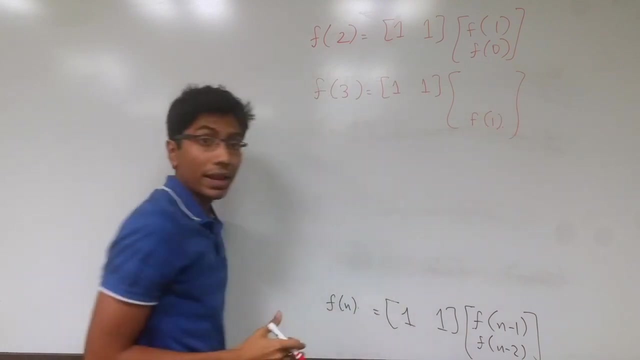 this matrix: f of 1 and f of 0. So that's f of 2.. What is f of 3?? That's equal to 1 into 1.. f of 1 will come down, but f of 2 should come here, so rather we can just substitute this: 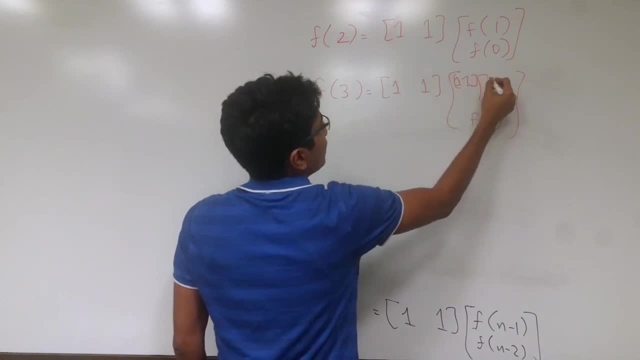 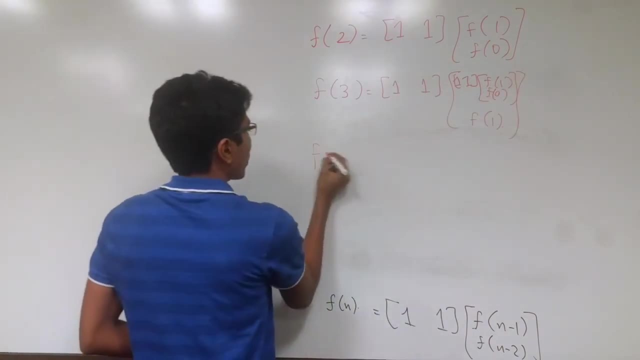 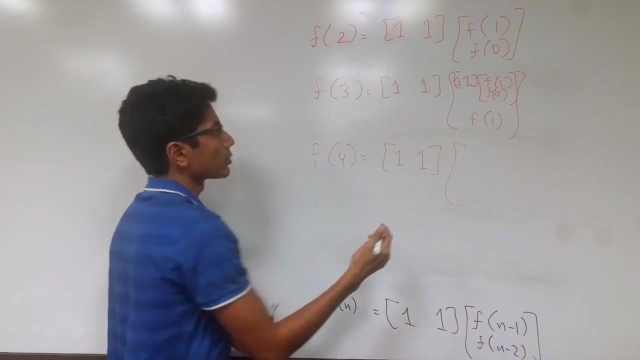 So that is 1, 1 in this tiny matrix that I'm drawing, But it's not important, we are actually not going to be calculating these terms. Okay, that's, that's another thing. What about f of 4?? This is 1, 1 into f of 3 and f of 2 are the two terms. 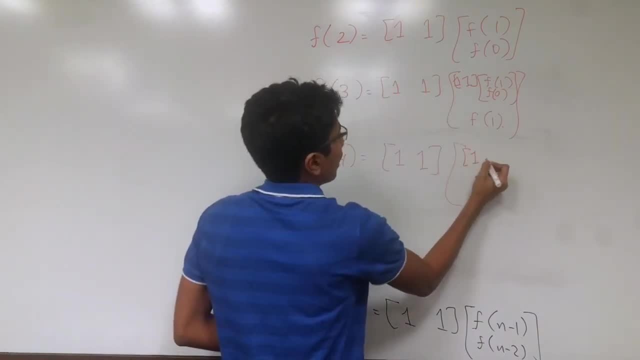 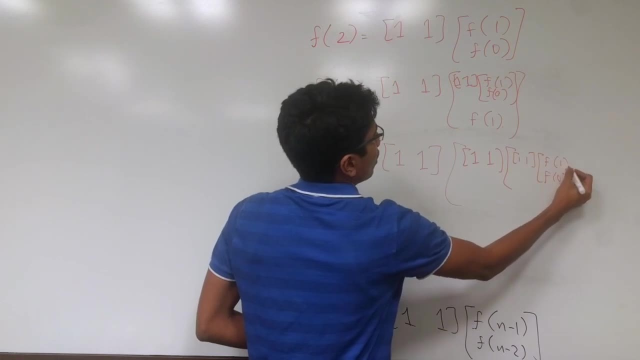 which should come. So I'm going to take f of 3 here and this big big equation is actually going to come out: 1, 1, f of 1, f of 0.. That completes the first term, In fact. 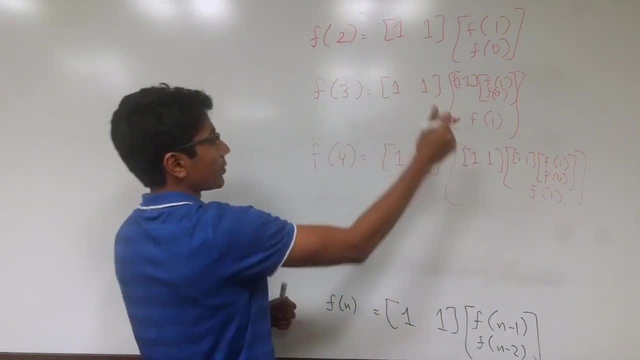 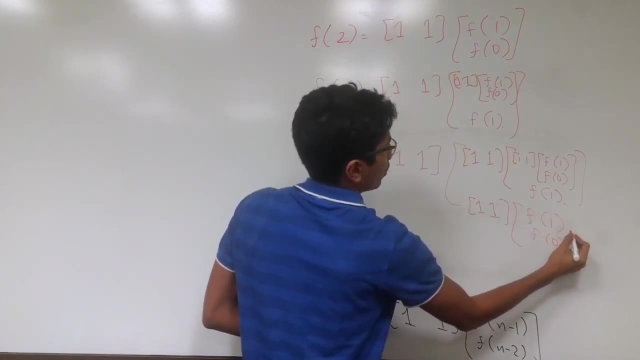 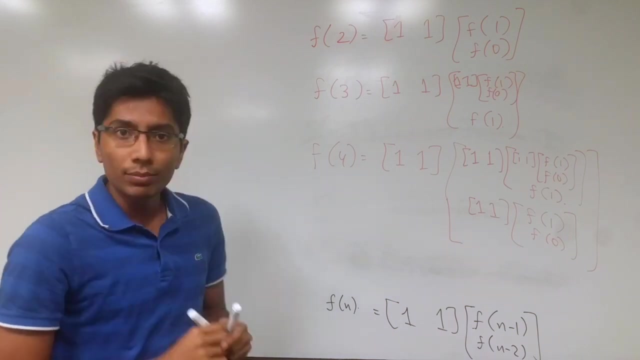 it still doesn't. so there's this term down Now. that completes the first term, and we have f of 2 below, Which is this term. This entire thing is just f of 4.. But there is something important to notice. 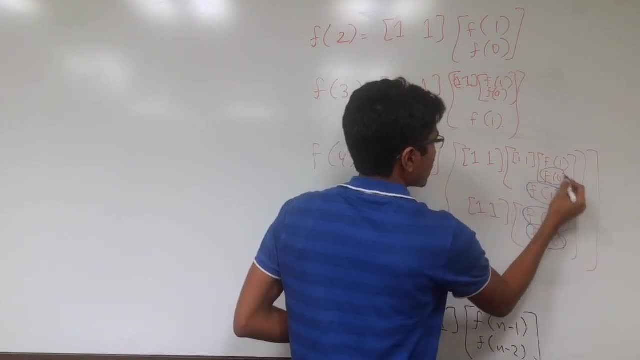 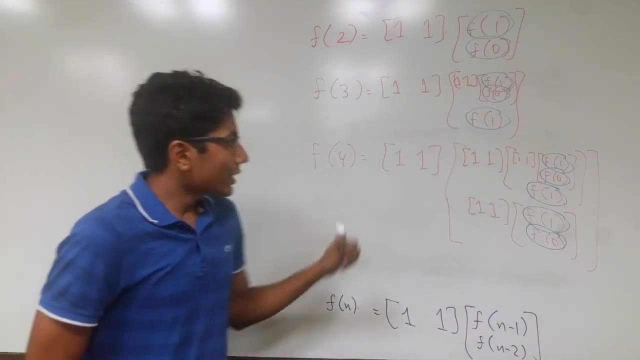 Look at these terms: f of 0, f of 1, f of 1, f of 0, f of 1.. And you don't see any other terms here. you just see the two base conditions here. So what this gives us is an idea that any Kroganaki number can be represented using the. 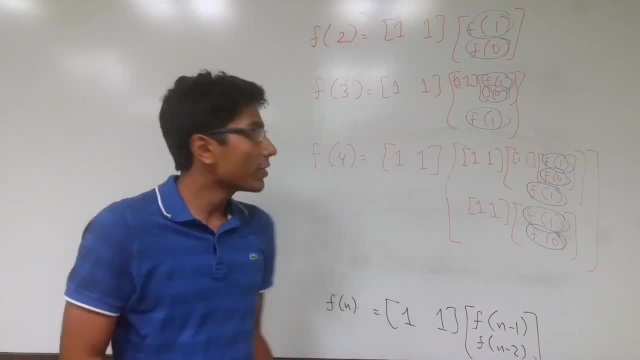 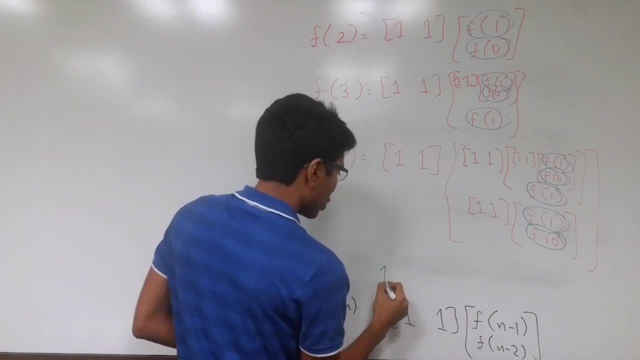 the base conditions, But our math is still not good enough. We have taken a vector and tried to multiply that with another vector. So these two are matrices, but we have a one cross two matrix and the other one being a two cross one matrix. A little more hard work. 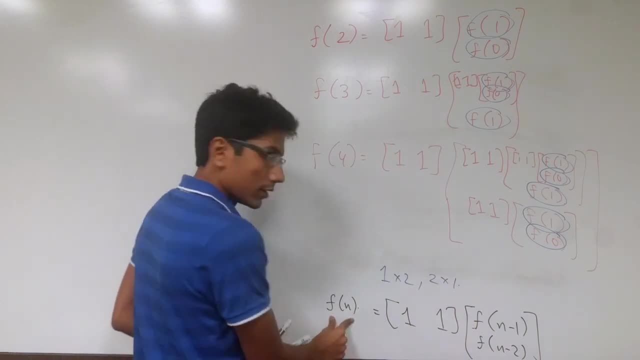 probably is going to give us this idea that f is nothing, but just taking another term, f, below, This being the matrix that we want. and to get that, this part makes sense, f. to get f, we just multiply this row with this column. That makes sense. What row do you need to? 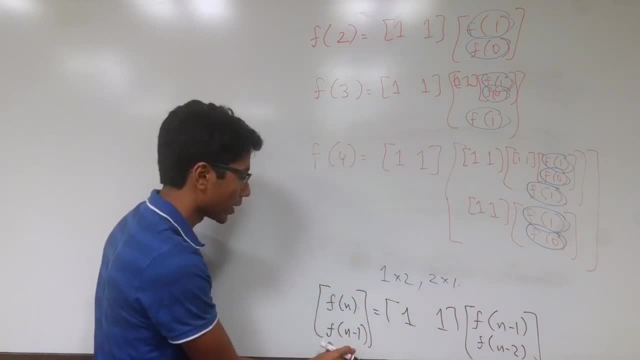 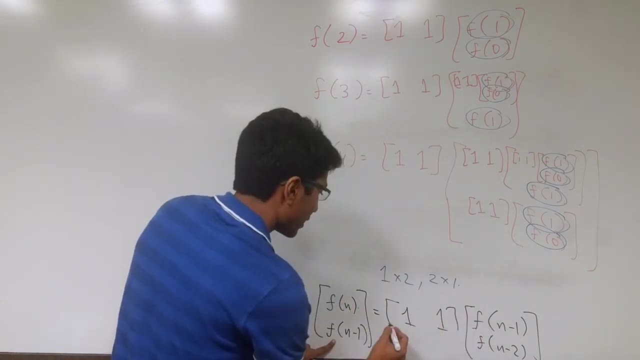 multiply with this column to get this term f. to get f, we need just this term, so that could be set to 1 and we can ignore this term, so that could work better. set to 0 and look at that. this row, when multiplied with this column, is going to. 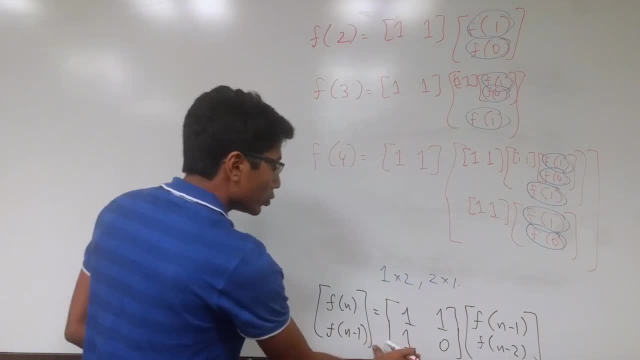 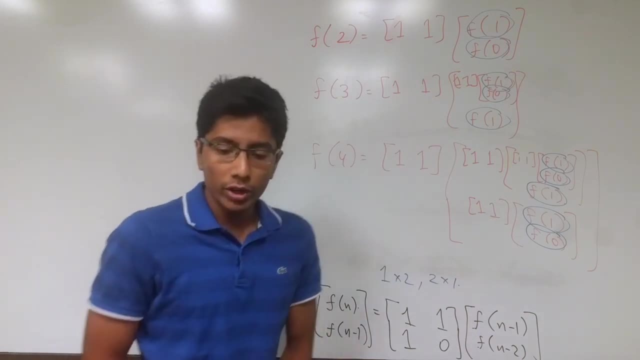 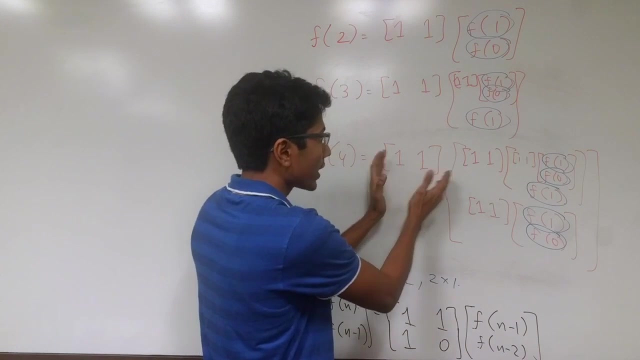 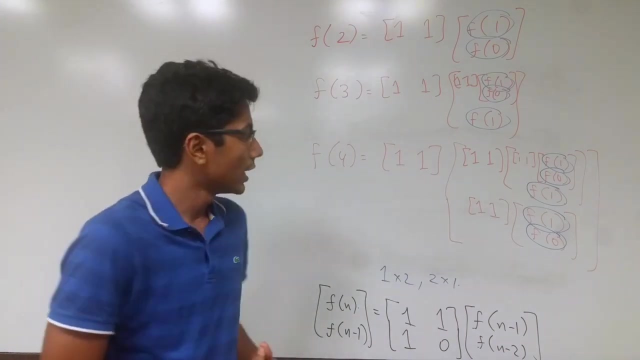 give you just f of n minus 1, which is what you need here. why did we do this? because the math is going to simplify over here, right? how is it going to simplify? look at this vector. can you find out its multiplication value with this vector or this vector, before you actually calculate these terms? no right. 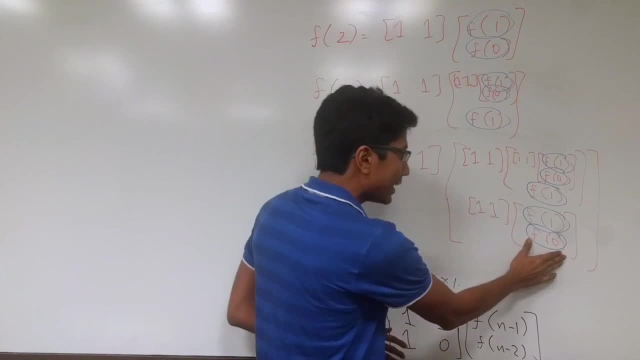 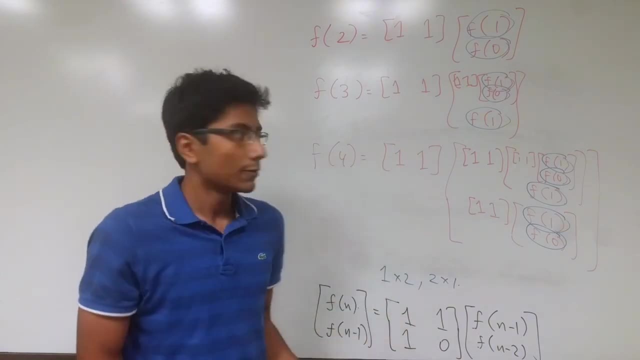 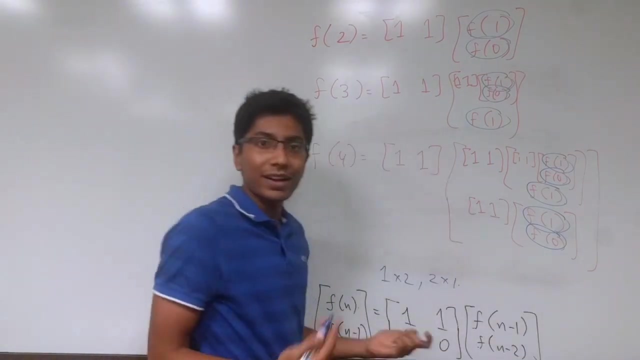 so whenever we have the base conditions with us, we need to multiply them with this vector to go to the next step, which is basically defeating the purpose of doing all this math, because if you're going and multiplying it with this vector, then that's an order n operation and you have a better algorithm for that. 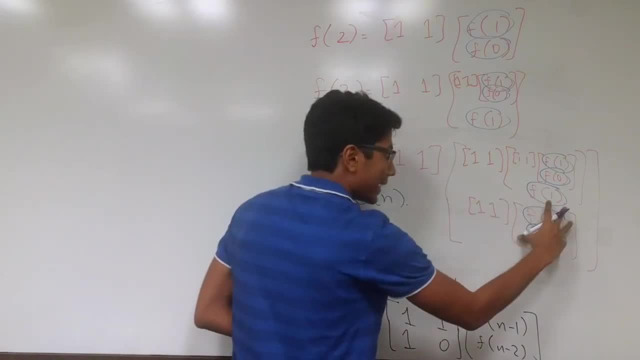 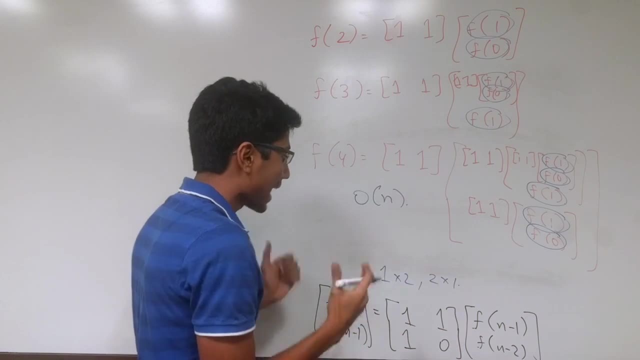 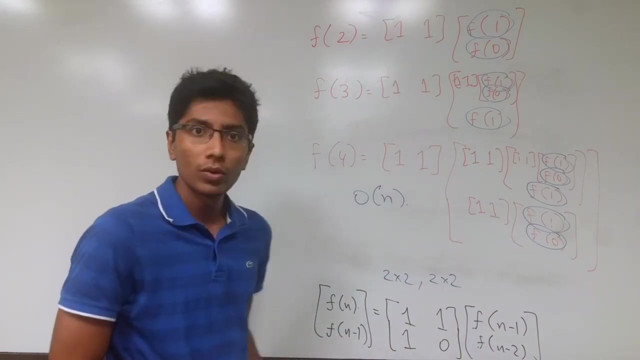 right. so this? this is nothing apart from give us the insight that every term can be represented using the base conditions, but this matrix representation is actually going to be making our algorithm very fast. How Well. this matrix is a 2 cross 2 matrix, meaning that you can take this matrix. 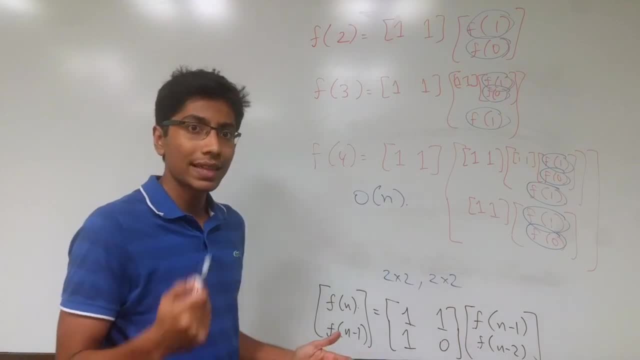 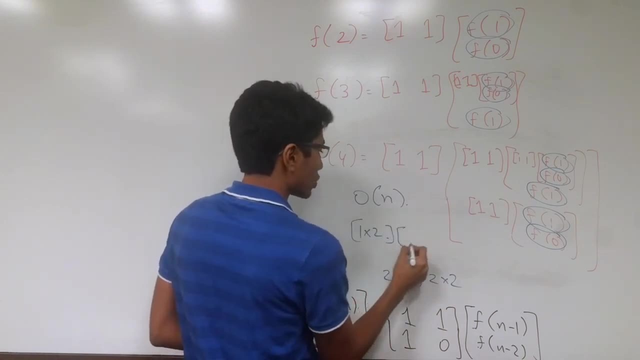 and multiply it with itself. That's the biggest insight. So earlier we had a vector of what 1 cross 2.. 1 cross 2 cannot be multiplied with 1 cross 2 matrices. Okay, the number of columns here has to be equal to the. 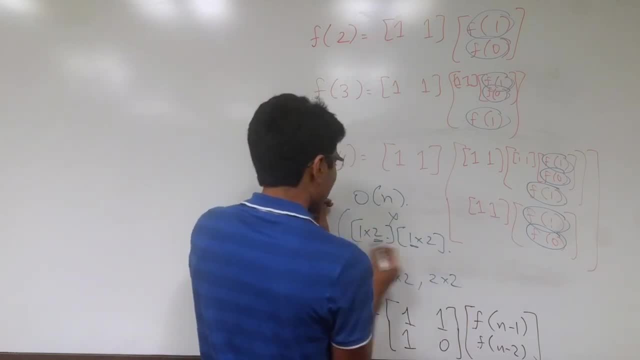 number of free flows of the second matrix. so this would not work. So whenever we are trying to actually put them together, the vectors together here, that wouldn't work because you would first need to multiply this with this and before that this with this and so on and so forth. so that will take too much. 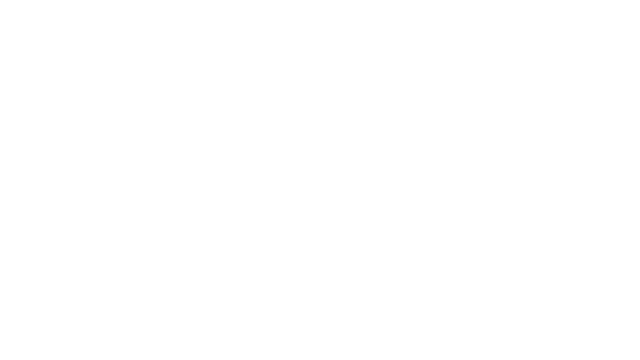 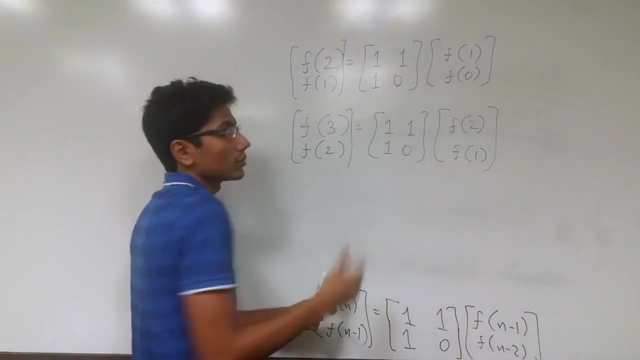 time. But here a 2 cross 2 matrix can be multiplied by itself. So now what we can do is take f of 2 and f of 1. as a column matrix and then represent that as a multiplication of two matrices. 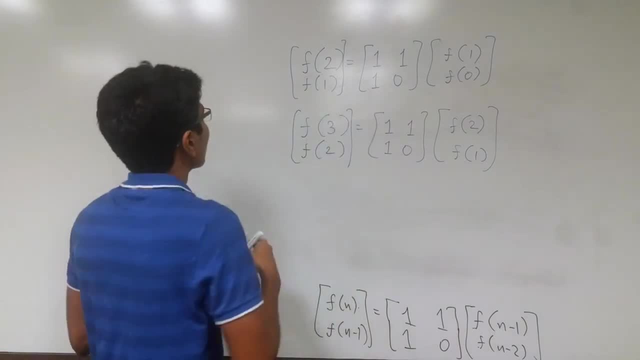 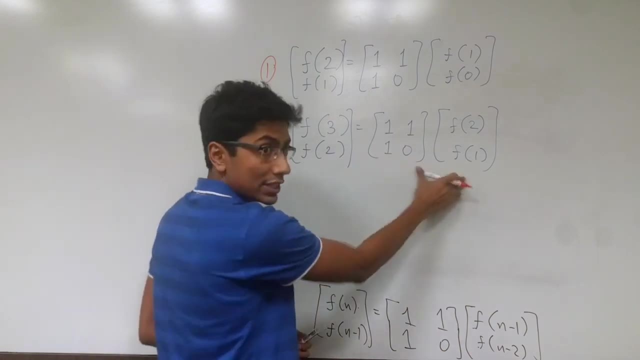 Okay, so this is our first equation, and the second equation wants to find out f of 3.. According to our equation, we also keep f of 2 and multiply these two matrices. But have a look at this matrix. This one can be substituted from the. 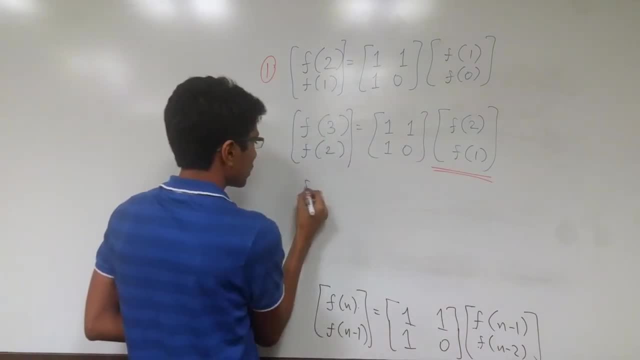 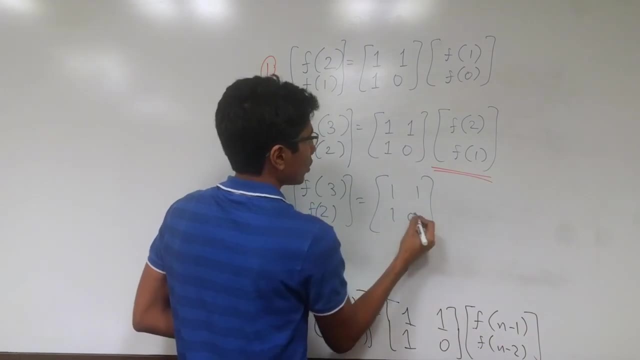 first equation. Let's do that. We get f of 3 and f of 2 as a column matrix being equivalent to 1, 1, 1, 0, and substituting we get 1, 1, 1, 0 and f of. 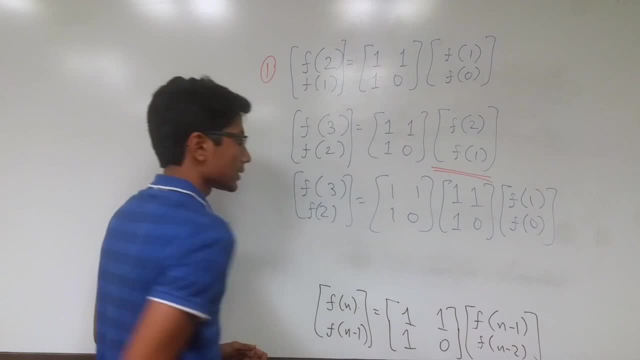 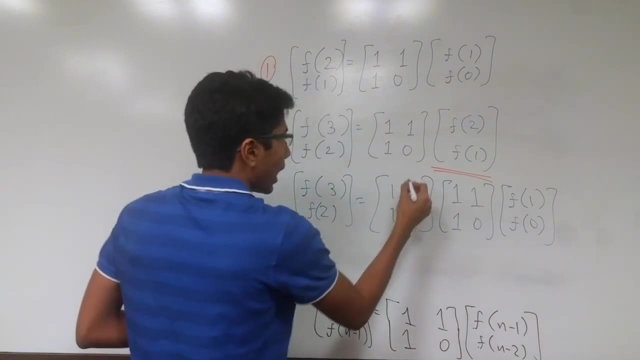 1, f of 0 being the column matrix. Here's the thing: You take these two matrices and you can multiply them. Okay, they are no longer. I mean, they are two cross two matrices, So the number of rows and columns are the same for these two. 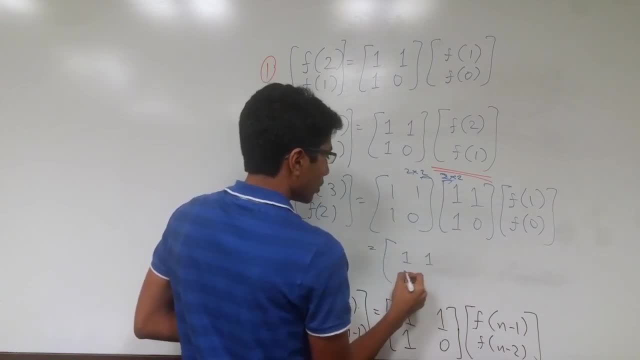 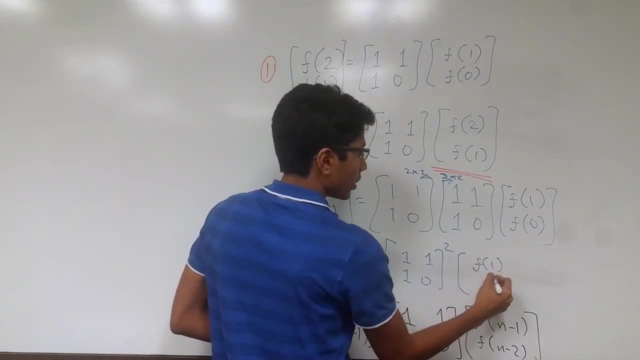 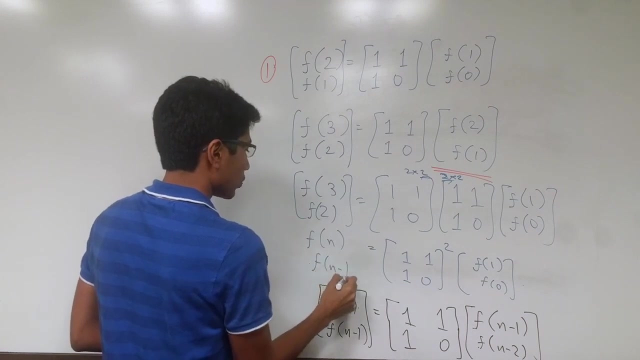 guys, That gives us a 1, 1, 1, 0 squared square. So this matrix has been squared and then we get f of 1, f of 0.. And in general, for the number f of n and f of n minus 1 being the column, you need n minus 1 as a. 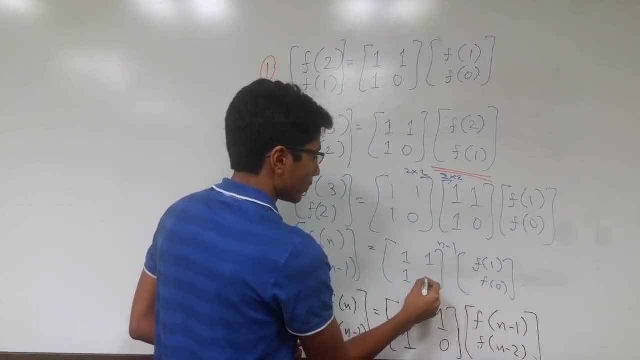 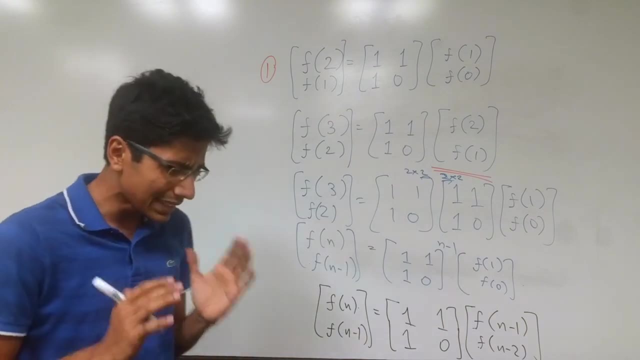 power of this matrix into f of 1, f of 0.. Okay, so that's how we can find the nth Fibonacci number using just these two terms. There is still a problem, though. We need to raise this to a power of 1.. We need to raise this to a power of 1.. So. 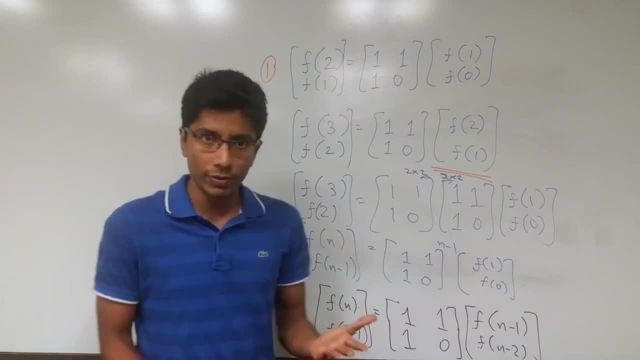 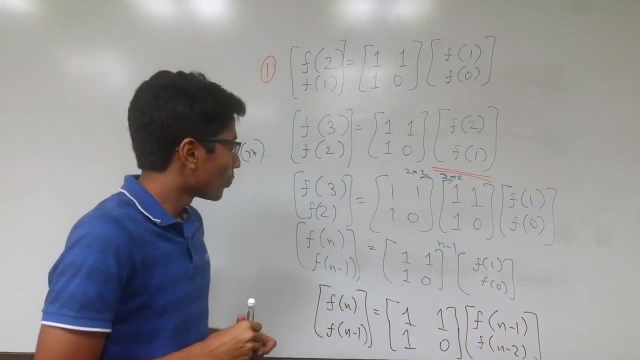 you need to raise this to a power of n minus 1. In the brute force way. of course, if you do this, it's going to take us order n time as bad as earlier, But we can do much, much better. So if you haven't seen the tutorial for fast, 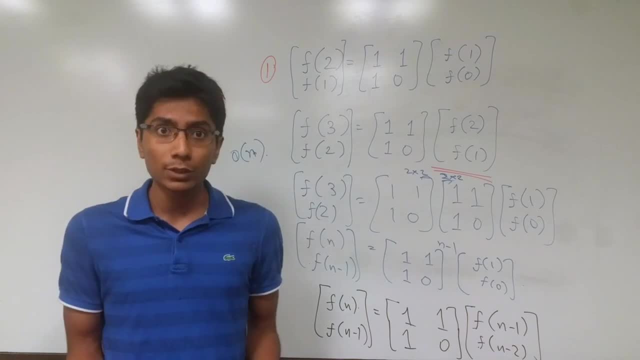 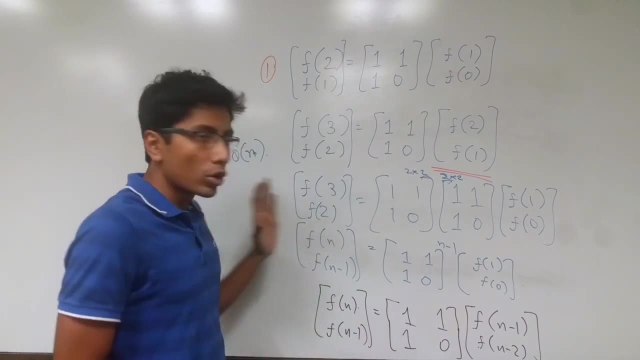 exponentiation you should. What we are going to do here is called binary exponentiation, So that is a little bit of that's the only part where there is actually dynamic programming here. But you could look at fast exponentiation It has. 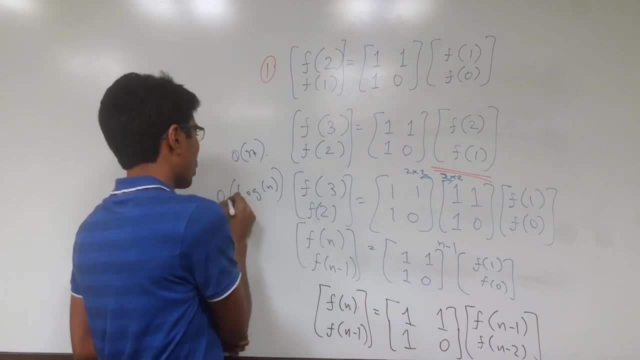 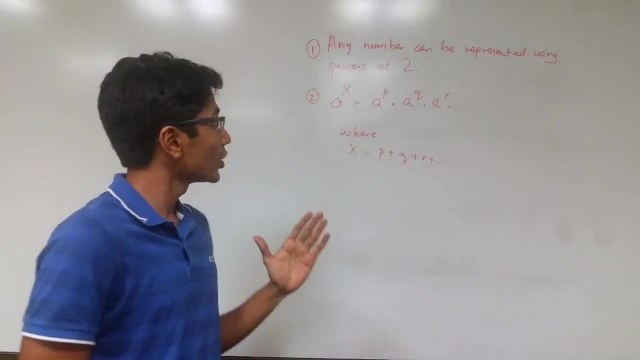 login time Time complexity. So that's as good as this one, but we're learning something new. this time Let's do that. So. binary exponentiation uses two main properties, the first one being that any number can be represented using powers of 2 or. 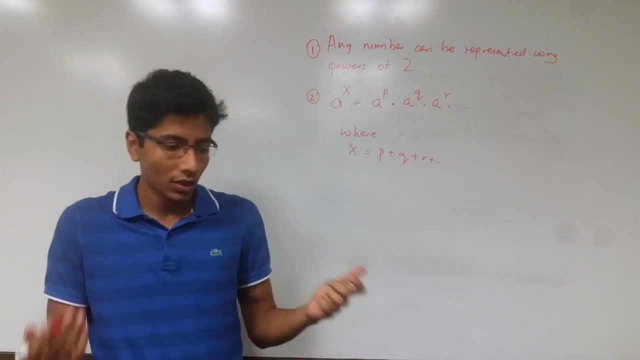 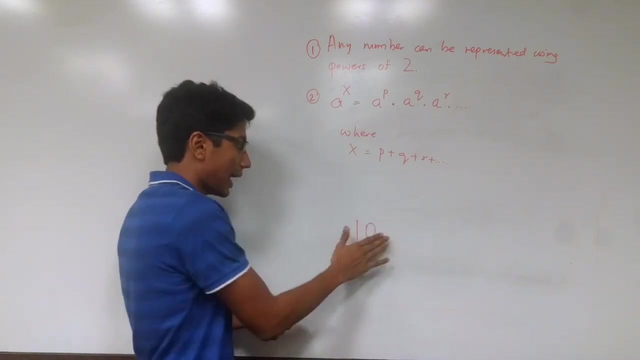 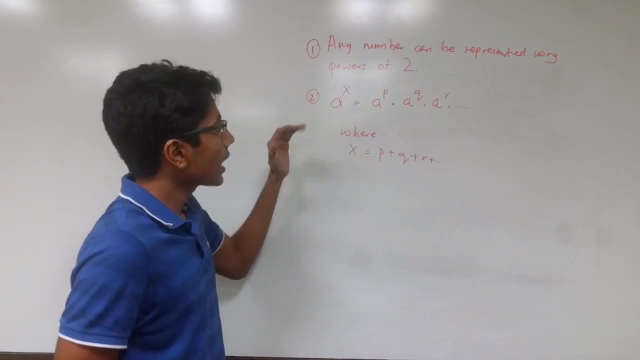 powers of 3 or powers of 4, actually as long as you have a good base System to play with. so decimal uses powers of 10 to represent any number, But you can represent any decimal number as binary also using powers of 2. That's one important thing to know. and the second thing is any number raised to the power X. 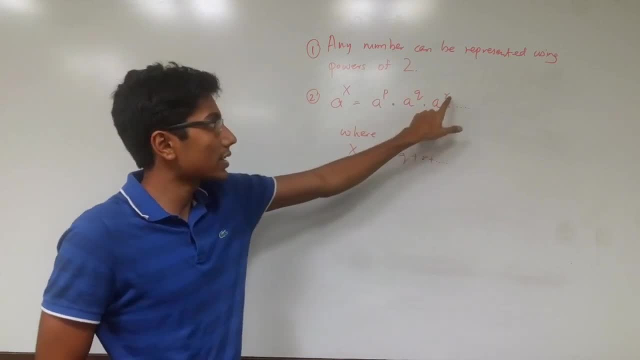 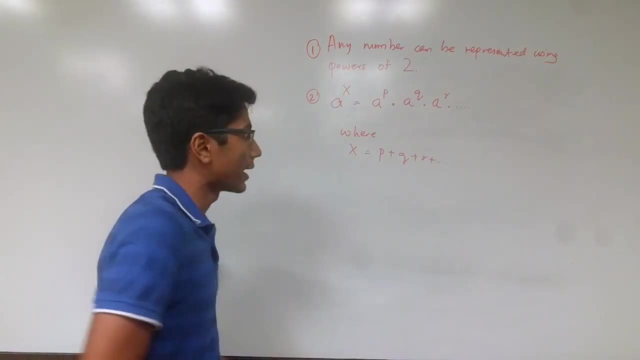 Is equal to a raise to power P, into a raise to power Q, into a raise to power R, Where X is equal to P plus Q plus R Plus, so on and so forth. So there's other exponents you can add here. So what we do is very clever. 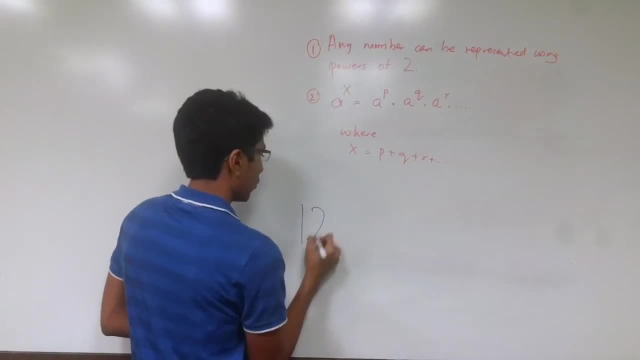 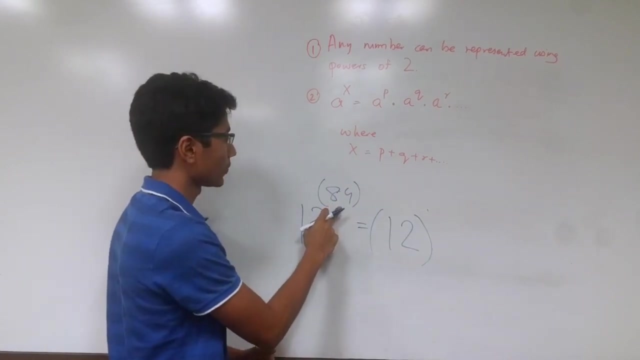 We take a number like 12 Having an exponent, let's say 84, and We break this exponent into powers of 2, So that is 12 raised to power. What should be 1,, 2,, 4? Well, we take the maximum power that we can from here, So 64. 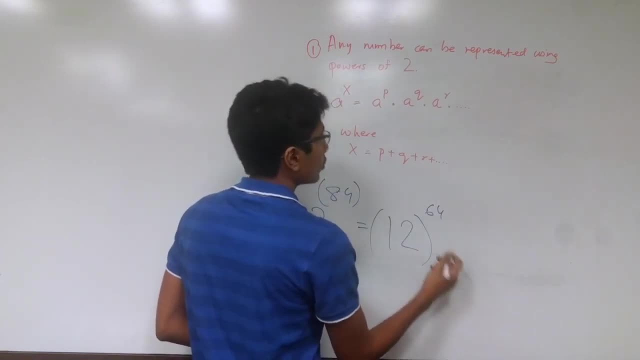 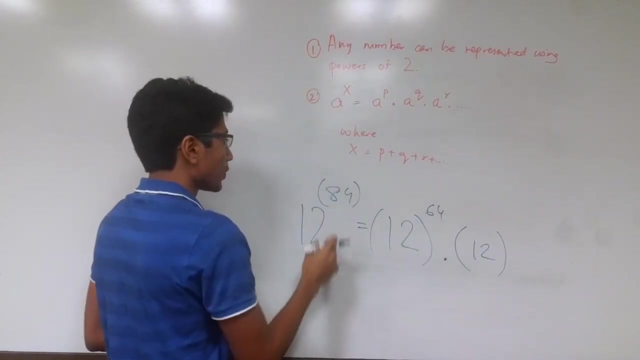 12 raised to power 64. that's, that's nice into. This is what we are doing, Right, We're going in the RHS. So now again, you have to multiply by 12, because this is not equal to this. 20 is the power remaining. We want to take the maximum power from that, So that is 16. 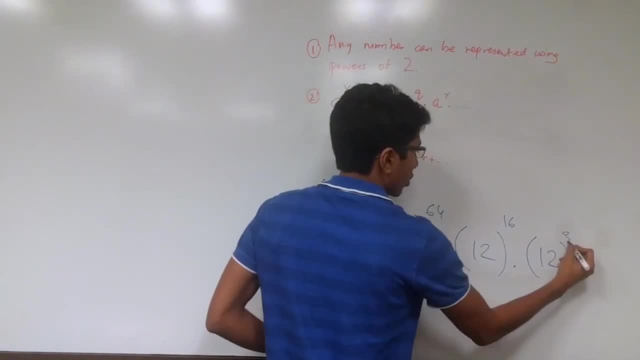 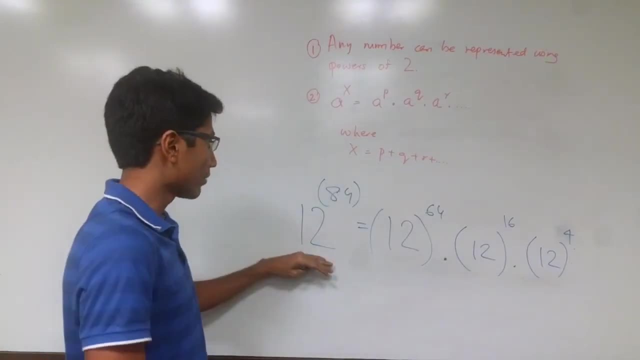 4 is the power remaining, which is itself a power of 2, so that is 12 raised to power 4. Now, what does this give us? Three terms, and we have this number. Why do we take this number and break it into three terms at all? 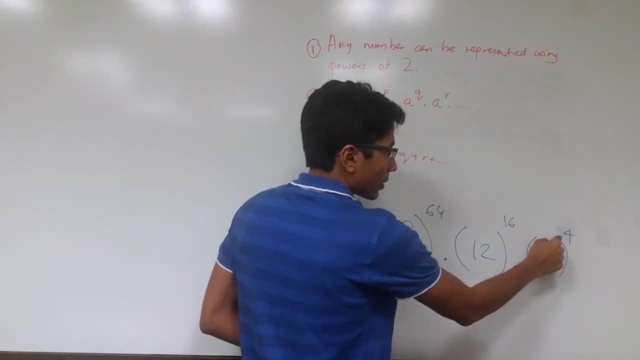 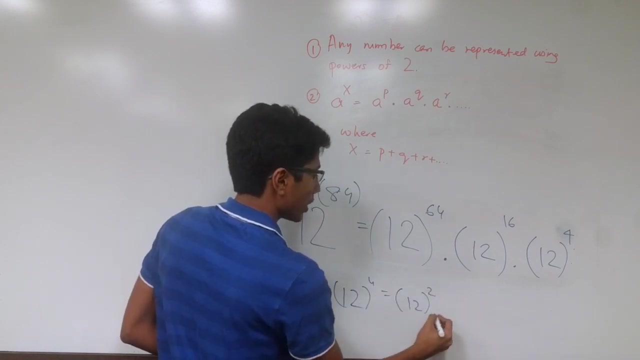 because to calculate 12 raised to power 4 Is like calculating 12 raised to power 2 into 12 raised to power 2, Which in turn, 12 raised to power 2, can be calculated using 12 into 12. Now 12 raised to power 16. the same thing can be done here. 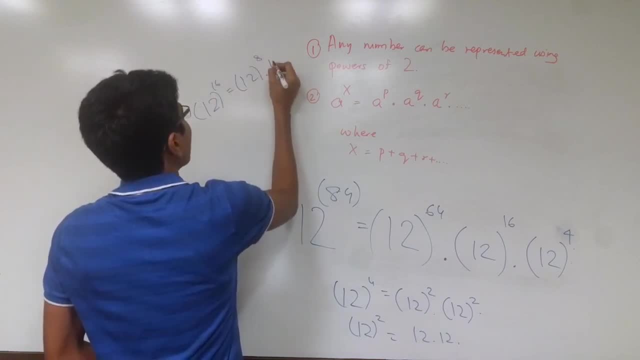 12 raised to power 16 is like calculating 12 raised to power 8 into 12 raised to power 8. That, in turn, can be done using 12 raised to power 4 into 12 raised to power 4, which you have already calculated here. 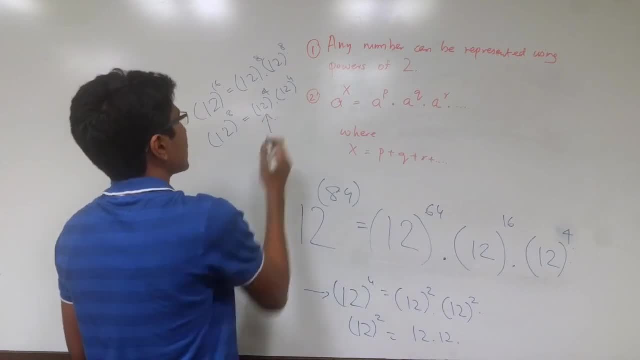 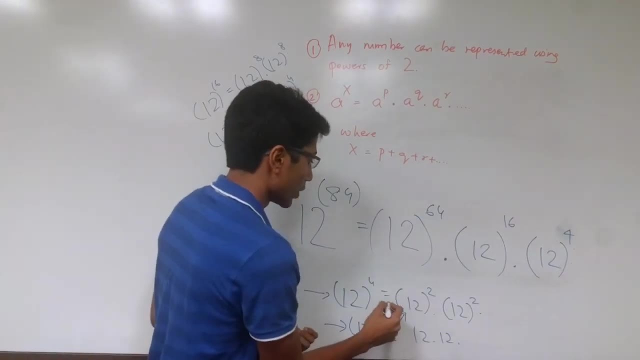 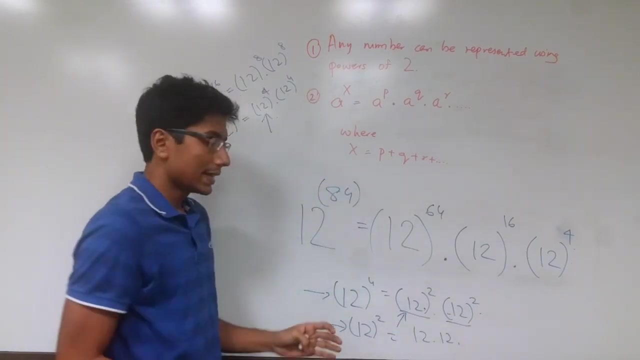 So this and this are the same. now, of course, You're seeing that there's a lot of common stuff happening here, and this is nothing but a recursive equation, where your function is nothing but multiplying the two results, and once this is calculated, you don't need to calculate this again. This is where the dynamic 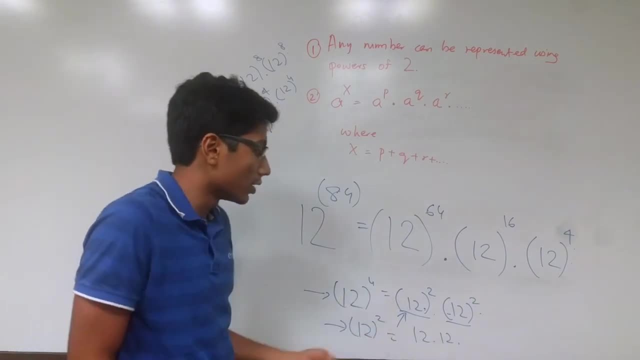 programming comes in. It's a very simple way to do the dynamic programming here, because it's a very common and intuitive way and you don't need to think of many results. but let's start off simple and what's happening is you're taking the two results that you have, multiplying them and making bigger and 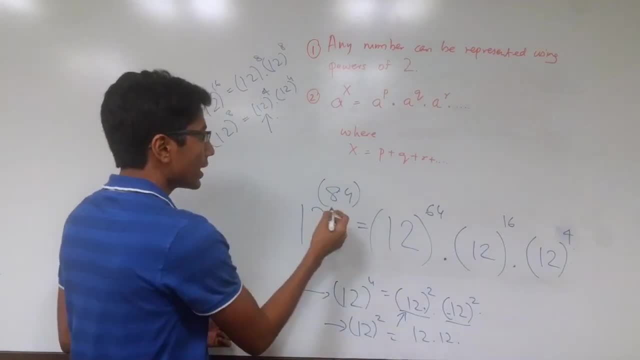 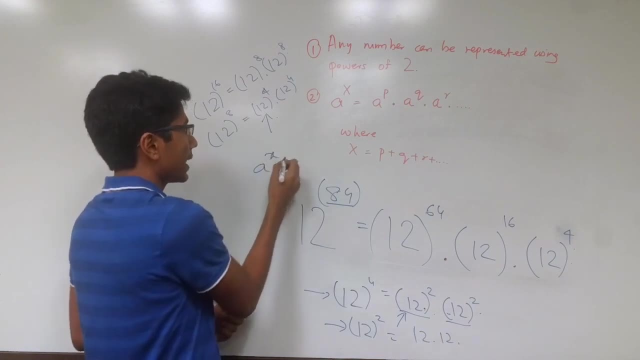 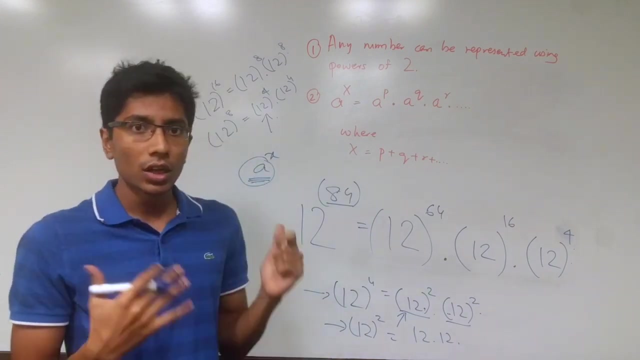 bigger powers of two. using that, and now, because we know that any number can be represented as powers of two, we can find a number, a raised to power. any number, okay, as long as you have all the powers of 2 of a. So that's the strategy Now for 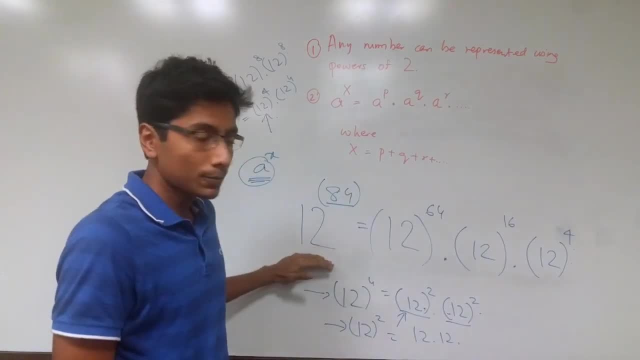 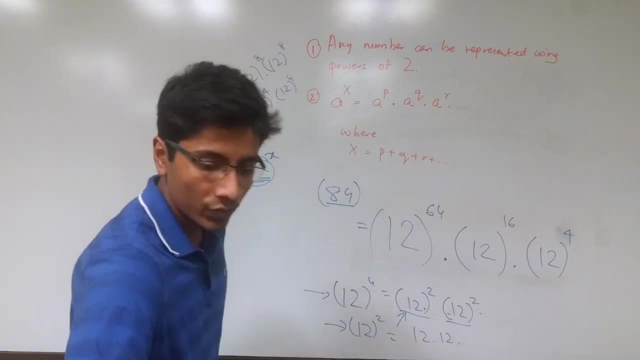 Fibonacci numbers. how is this going to help us? We are going to do the same thing, the same logic of binary exponentiation, using matrices. So instead of having a simple number here, we are going to be having an entire matrix here. the matrix Is this: 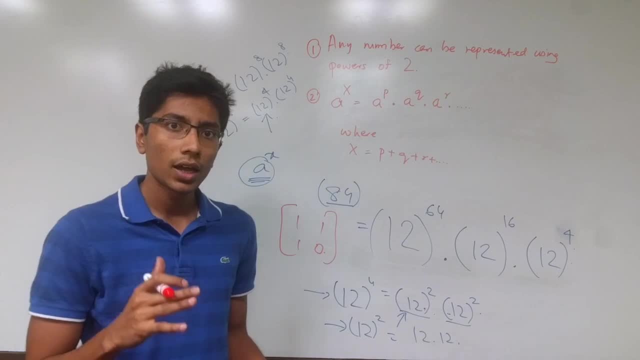 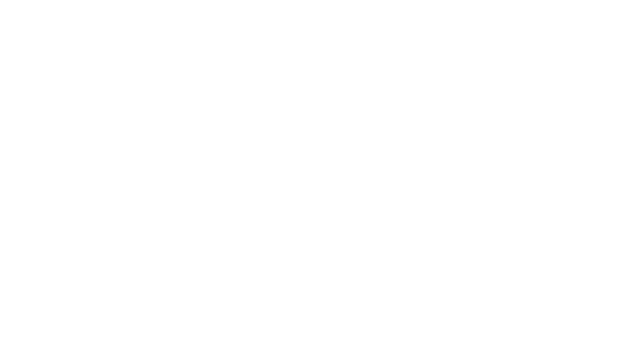 going to work on matrix exponentiation also the same logic? Yes, it will, because matrices are. I mean, when you multiply them they are associative. So it works. As an example, F of 14 is equal to this matrix that we found, raised to power 13 and the 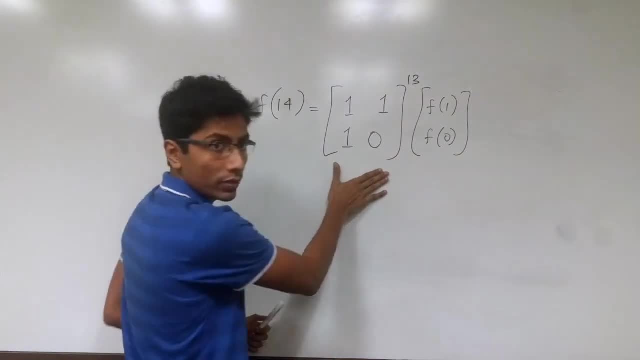 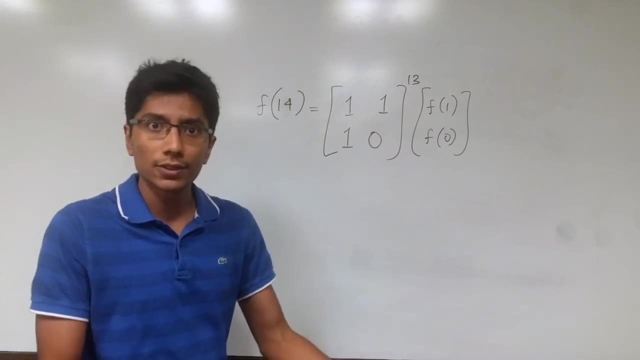 two base conditions as a column. So this is the core of the problem. right, Let's do binary exponentiation on that. but before doing that, of course, we need to keep all the powers of 2 stored with us for this matrix. So the first power of 2 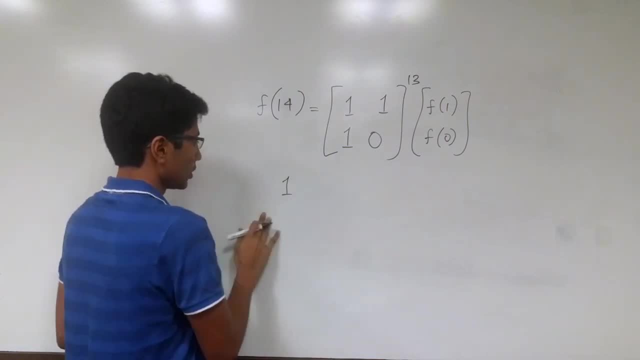 we can think of is: 1.. Okay, 2 raised to power 0 gives you 1, so that's also power of 2.. 2 raised to power 1 gives you a power of: gives you the result of 2.. 2 raised to power 2. 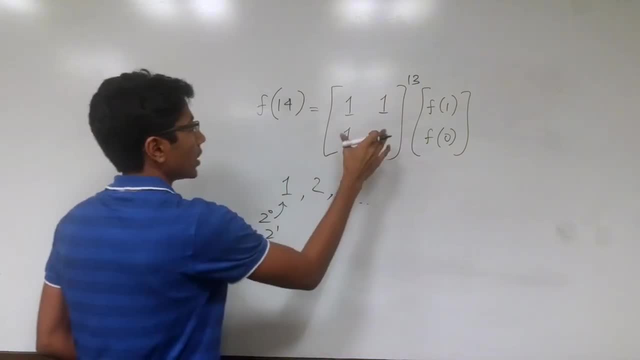 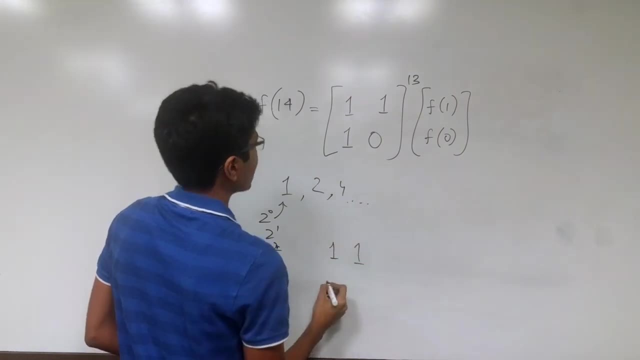 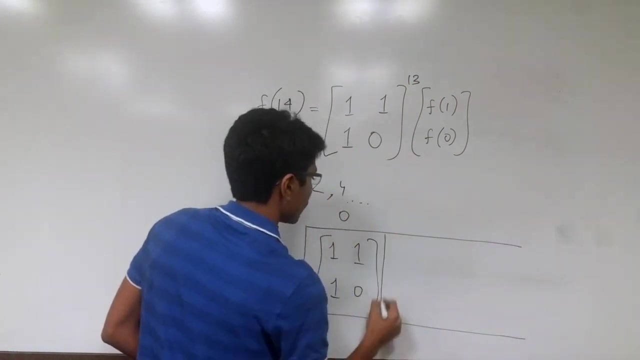 gives you 4, and so on and so forth. So these are the powers. we need to store This matrix raised to power 1, what does that give you? Well, it gives you a matrix itself. Okay, so this will be stored at index 0 in our storage array. 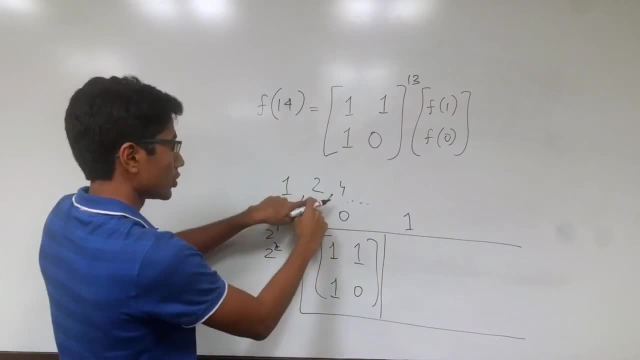 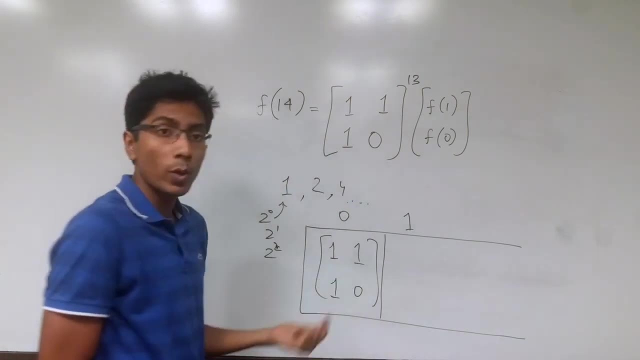 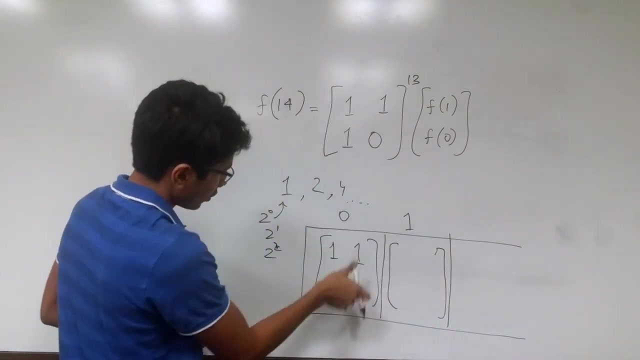 At index 1, we need this power, which is 2.. So that is this matrix squared. How do we find that? We multiply this matrix with itself. So that's going to give us a result and we're going to calculate that on the spot. So this is multiplied by: 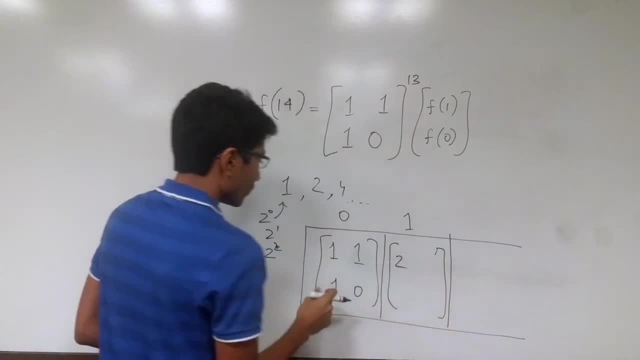 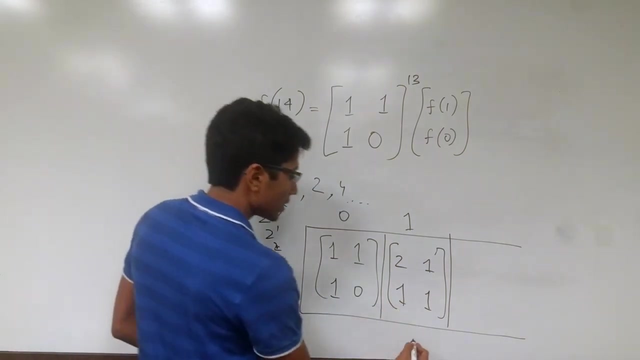 itself. So that is 1 plus 1, this is 2.. And the second column will be 1.. The next row, so that is 1 here, and 1, 0, so that is again 1 here. So this is the second entry you have, which represents. 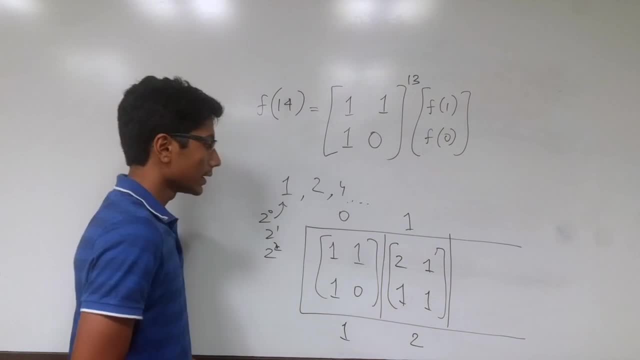 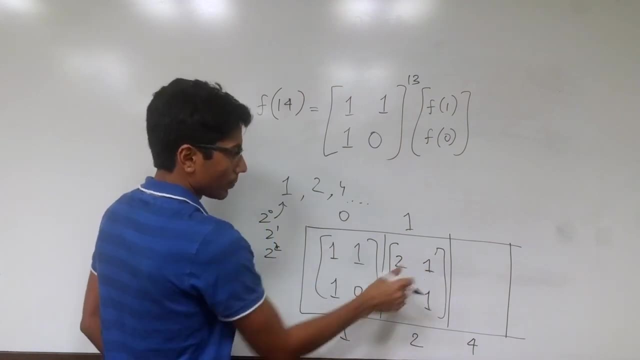 power of 2, this is 1.. Now 4 has to come in. So this matrix raised to power 4 will come in immediately now, which is this row with this column, gives you 4 and 1. So that is 5.. 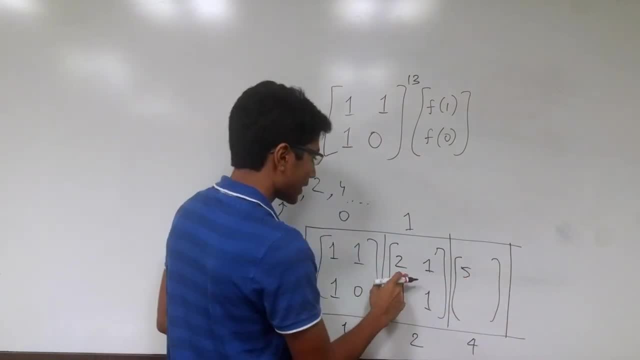 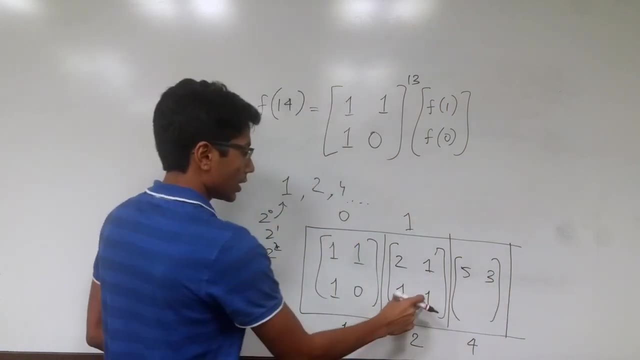 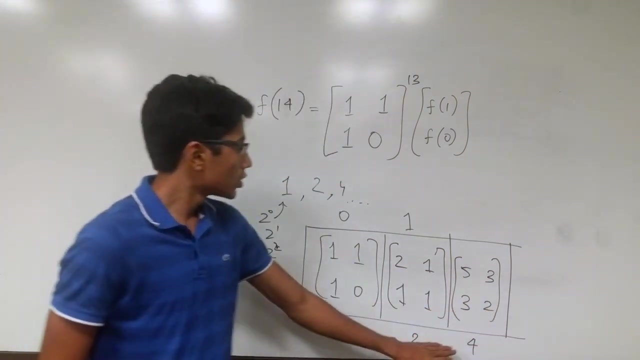 This looks like a formulaic term, by the way, and that makes sense. So 5 with the next is going to give you 3.. This one with this gives you 3 again and finally, this gives you 2.. So this matrix raised to power 4 gives you this matrix: 5, 3,, 3,, 2.. 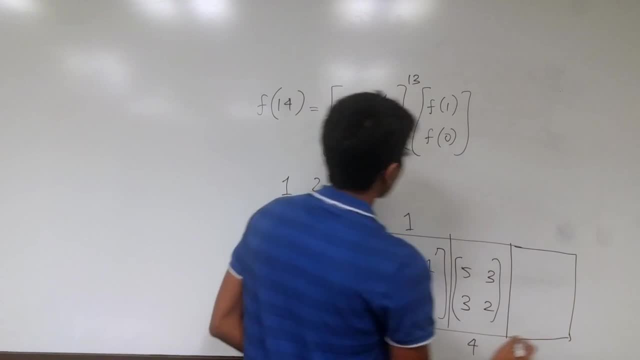 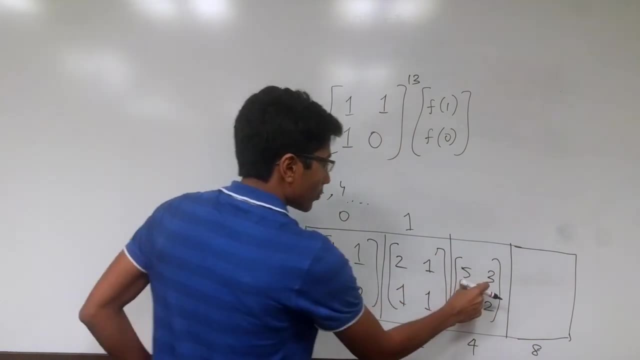 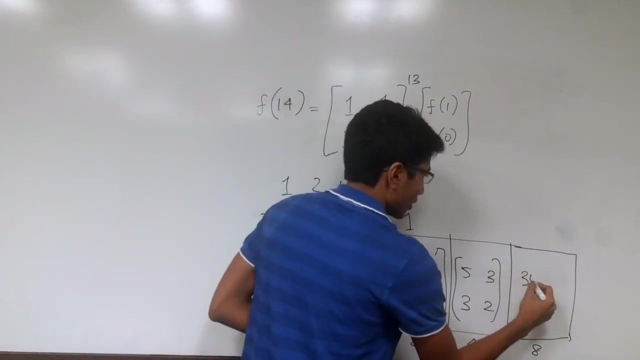 And let's take one final entry. I think that should do it. Yeah, 8 should do it. So that's 5.. 5, 3 multiplied with these two is going to give you 25 plus 9, which is 34.. God, I hope I'm right. What else? Well, 15. 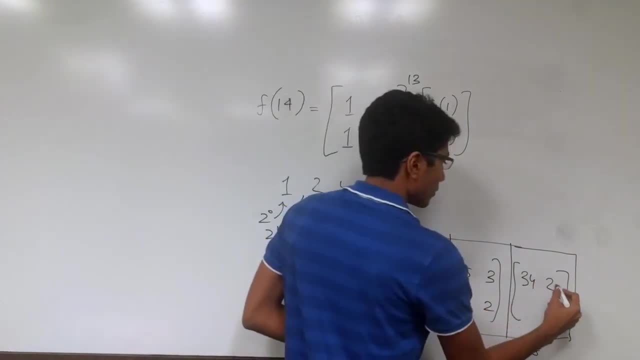 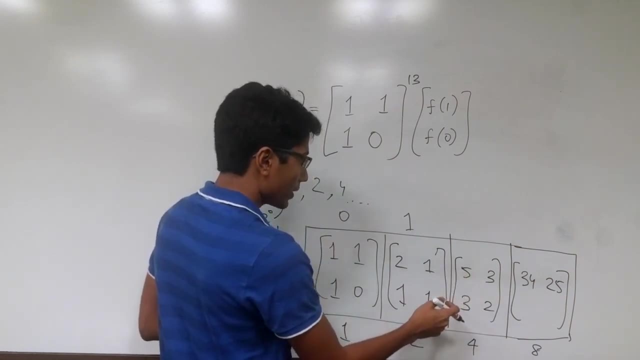 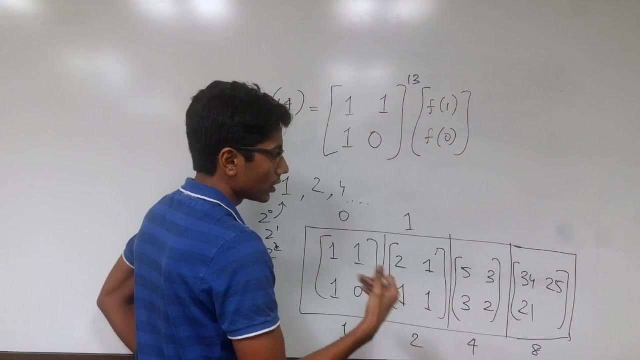 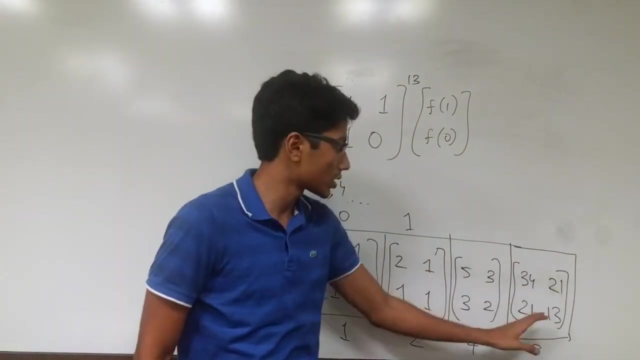 plus 10.. So that is 25.. Now these two multiplied with this, So that is 6 plus 15, which is 21.. And this with this, so that is 9 plus 4, so that is 13. okay, in fact this is 21 because this. 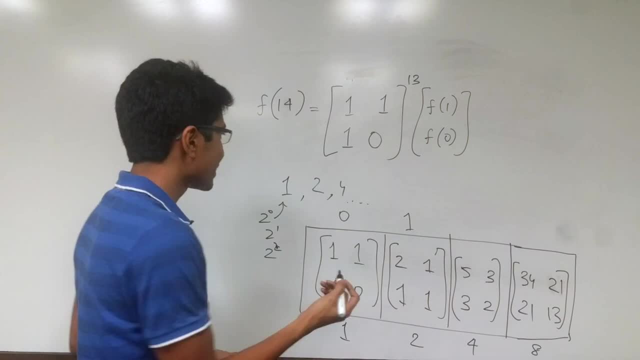 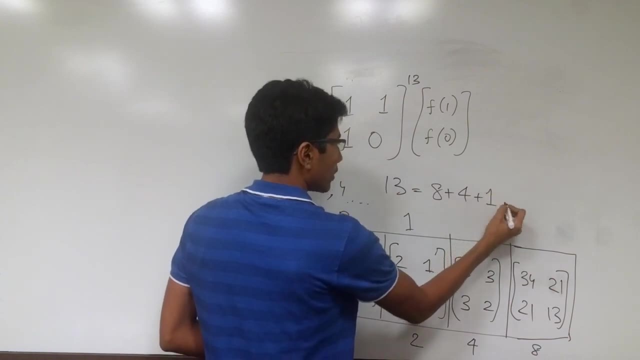 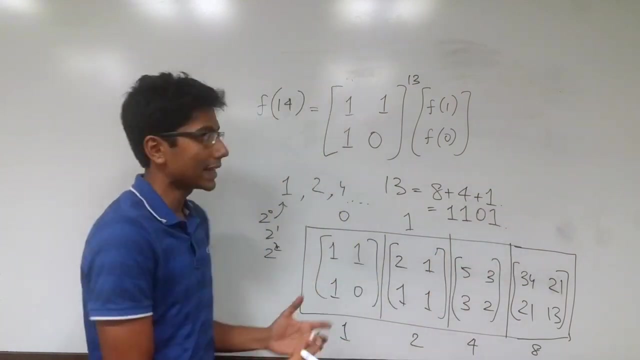 matrix has to be symmetrical. and now what we do is represent 13 as powers of 2, so that is, 13 is equal to 8 plus 4 plus 1. now, if you look at the binary representation of 13, that is 1, 1 0, 1. this makes sense, because, had this been? 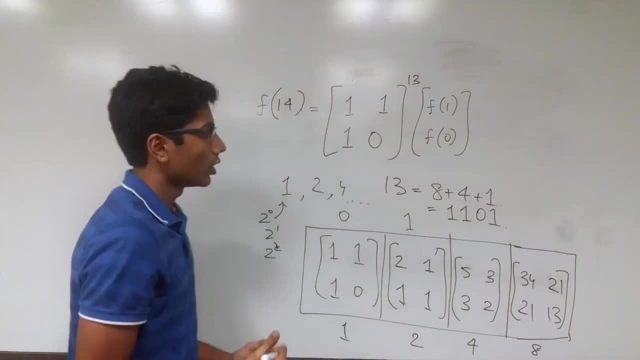 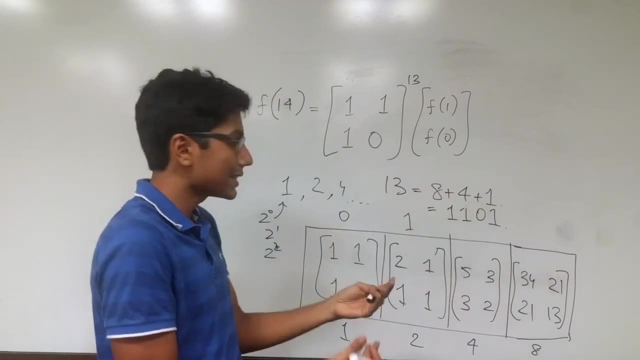 set to 1, you would had a plus 2 here. okay, you are representing 13 as powers of 2, and that's why in the binary representation, every bit which is set means that a number of that power- 2 raised to that power- has to be added to. 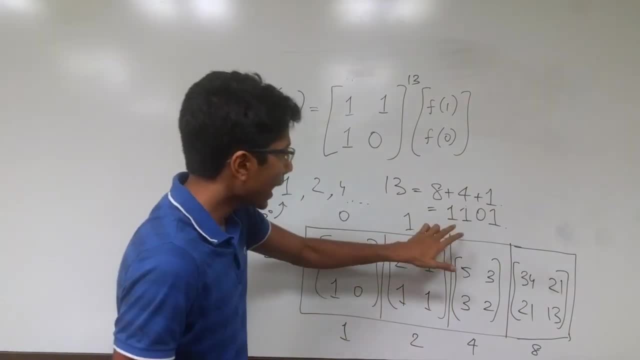 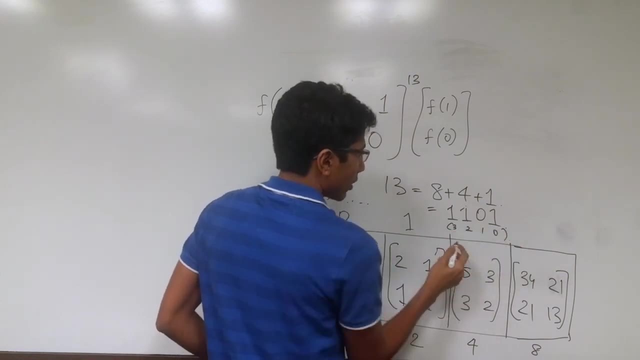 get this number. so basically, what we want is if the binary bit and that index is set. so this is: index is 3, 2, 1 and 0. so if the binary bit and that index is set for the exponent, so if the binary bit and that index is set for the exponent. 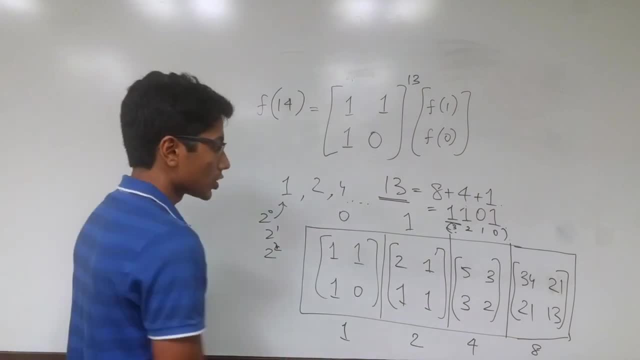 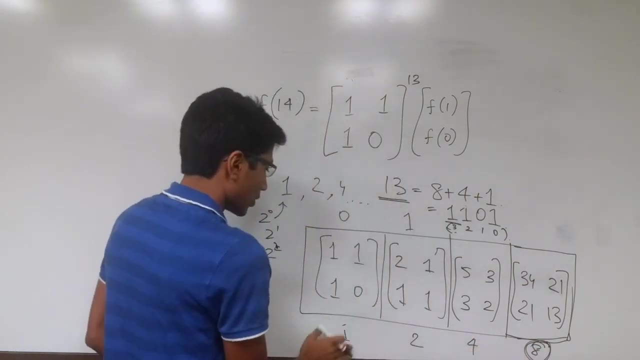 that means that the matrix has to be raised to that power. so you take the power of the matrix and that position. okay, at 8. so of course in an array this will be 0, 1, 2 and 3. so at 3 is the bit set for 13. yes, so you need this power. 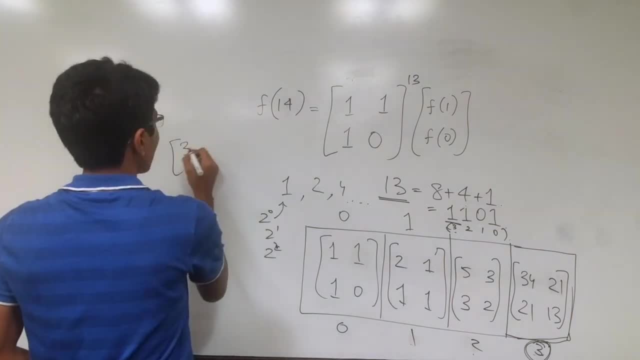 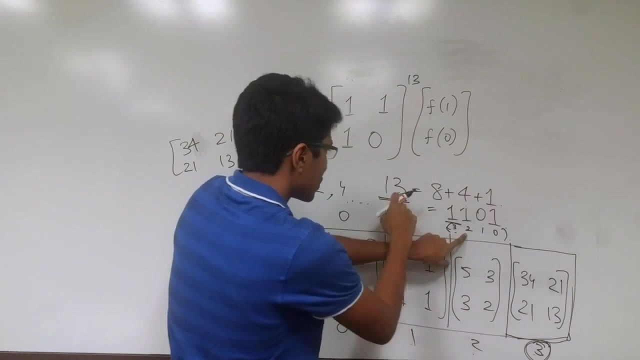 let's do that. let's take that as 34, 21 and 13. just write that a little neatly. yeah, this is one of the powers you need. what else at 2 is 13 having its bit set. yes, so this index is also needed. let's go. 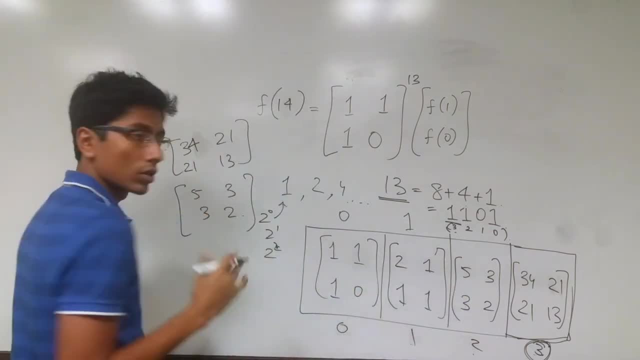 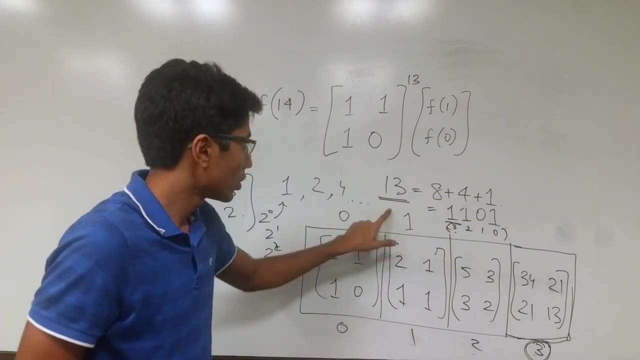 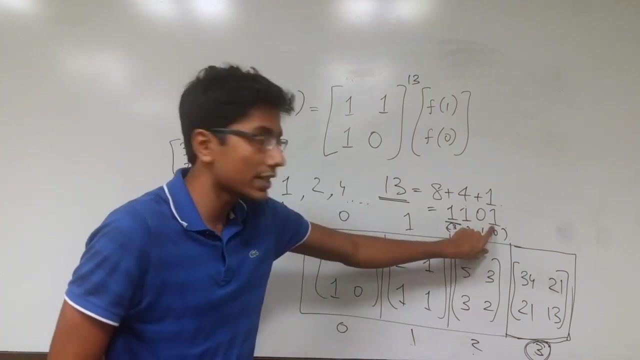 there, let's pick that up. 5, 3, 3, 2. this is also needed. what else? at 1 is the bit set: no. so do you need this power to raise your matrix to 13? no, you don't. one is not required, so we ignore that. what's the next thing? well, at index 0 it. 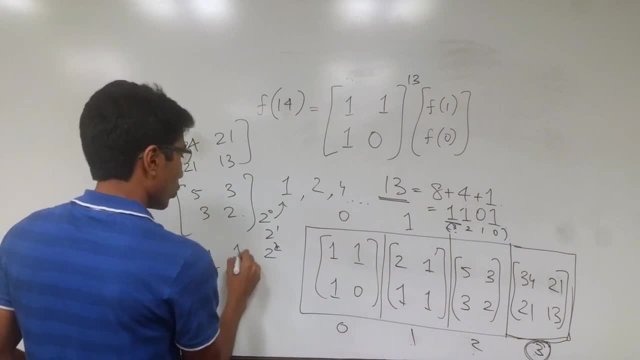 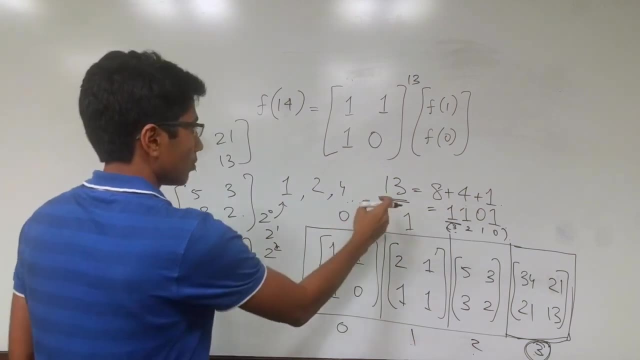 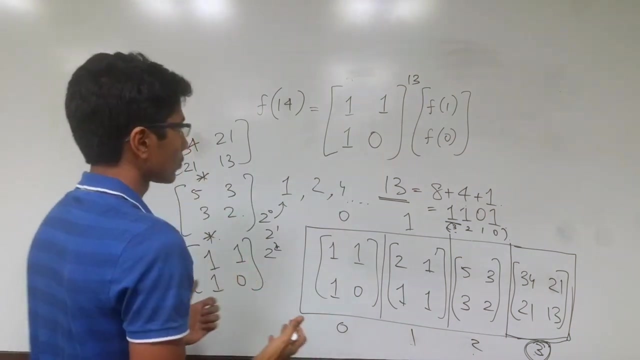 is set. so we pick this up: 1, 1, 1, 0. now these three powers are required to raise our matrix to 13. so what we do is we just multiply these three matrixes, because that's the thing about exponents: like we multiply them, then the 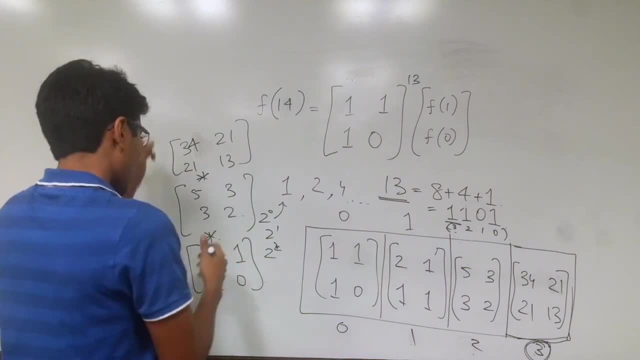 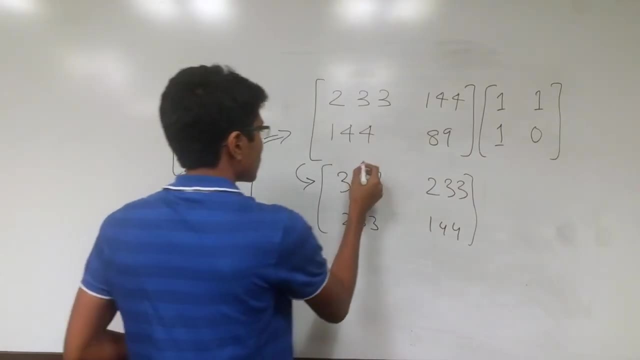 exponents get added right. so yeah, this one is going to get pretty complicated. I'll just fast forward to the result here. So that gives us a final result of 3, 7, 7, 2, 3, 3, 2, 3, 3 and 1, 4, 4.. Okay, but this is. 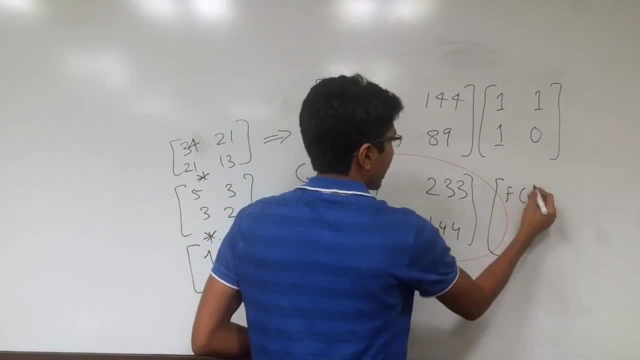 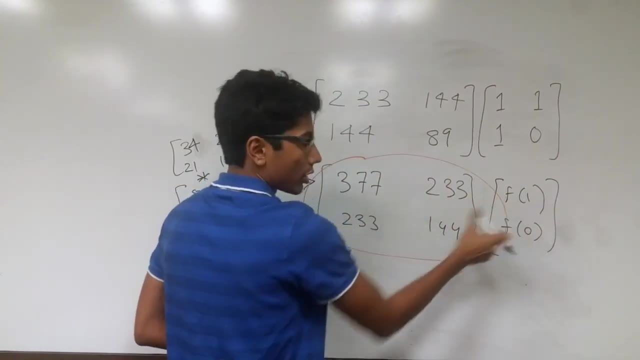 not the end of it. of course, There's a small procedure remaining. f and f have to be multiplied with it. Both of them are equal to 1 and 1.. So it's basically taking this row and multiplying with 1 and 1.. So that would be the sum of. 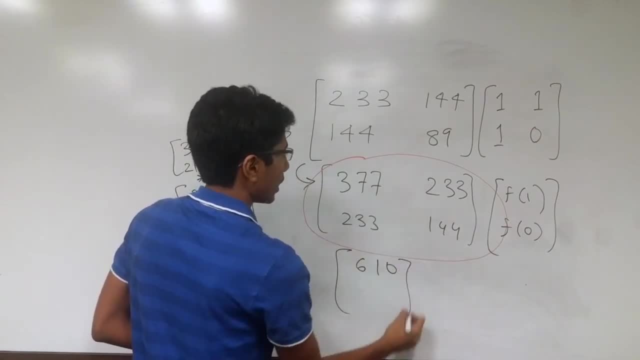 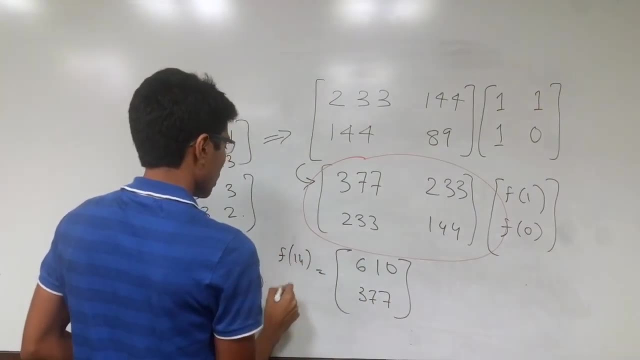 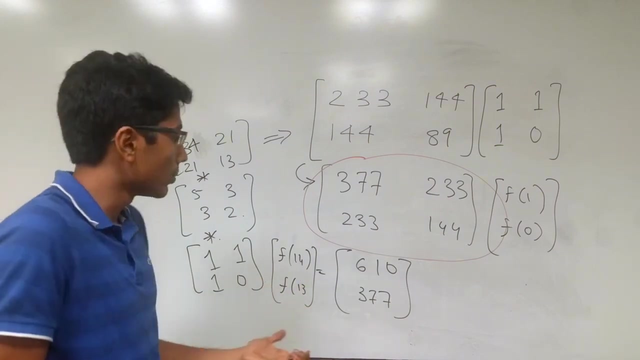 these two terms, which is 610, and this is equal to the second row, is equal to 377.. Okay, remember that this is equal to f of 14 and f of 13.. And so what we have done is find the nth term, the 14th term, of the Fibonacci sequence in log n time. 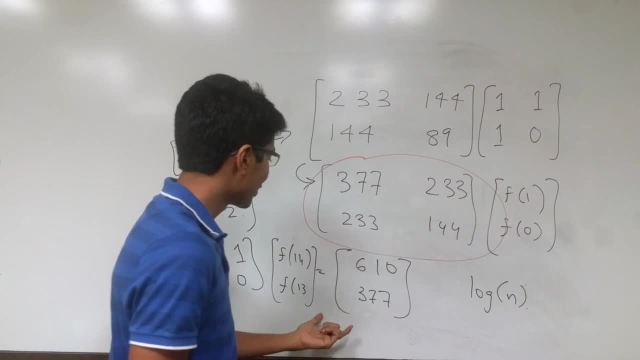 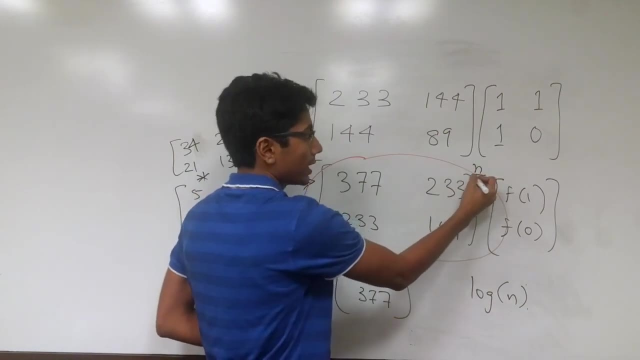 How's that? Because when you're taking that term, you know when you're taking this matrix and multiplying with it, you're going to get this matrix and raising it to a particular power. So whatever that power is, that will be order n power. And to get to this power you need just log n operations, because 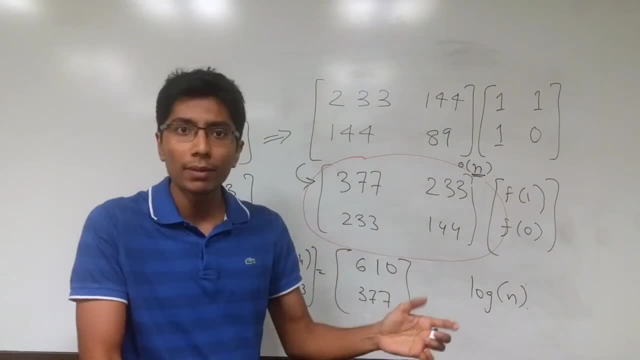 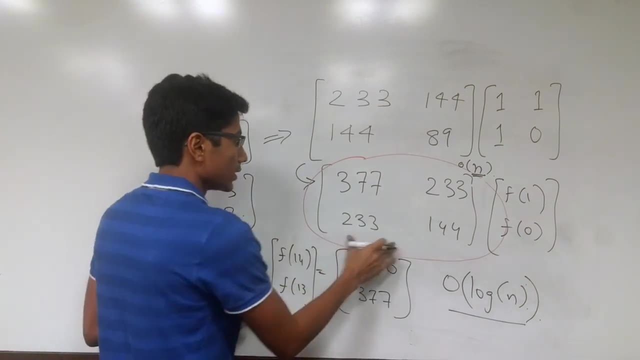 to represent this n, you need log n bits. So that's why the order complexity or the time complexity is log n. Okay, of course, we are assuming that matrices can be multiplied in order one time. But the thing is, this is a. 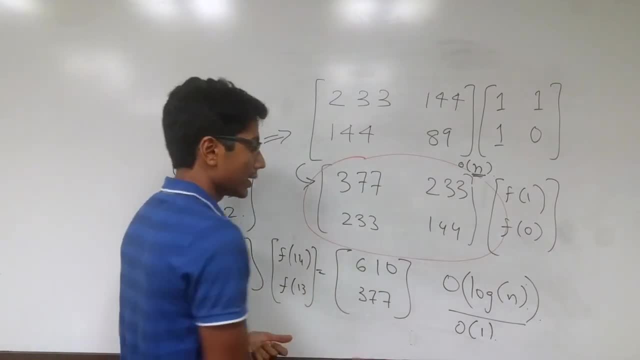 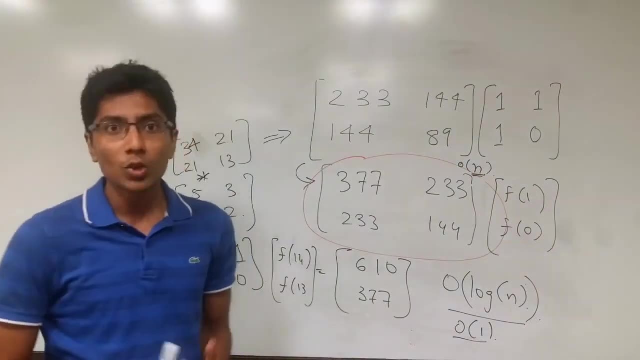 two-cross-two matrix To multiply with another two-cross-two matrix takes a very few computations. so that is order one. it's constant. So that's the reason why you have order log n time. So what we have done is find the nth Fibonacci number in. 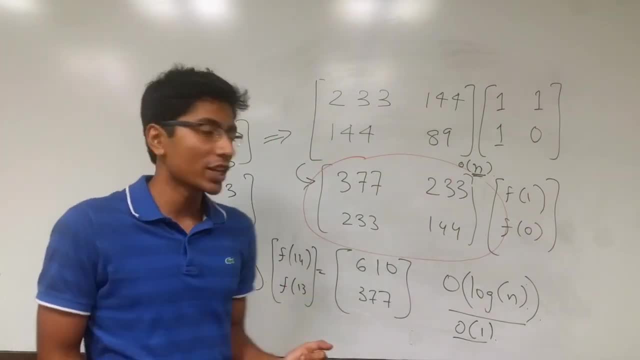 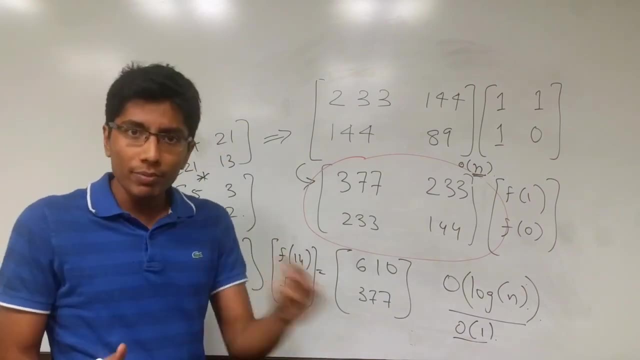 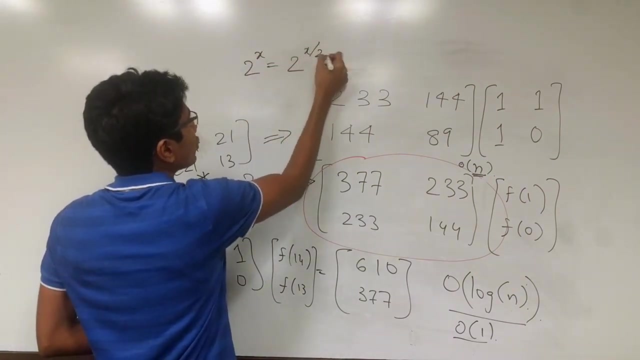 just log n time- and using binary exponentiation, which in turn uses dynamic programming. Now, where did the dynamic programming part come in? Well, it was so obvious that we might have missed it, so I'll just state it: 2 raised to power x. when we are finding this out, what we were doing is 2 raised to power x by 2 into 2 raised to power x. 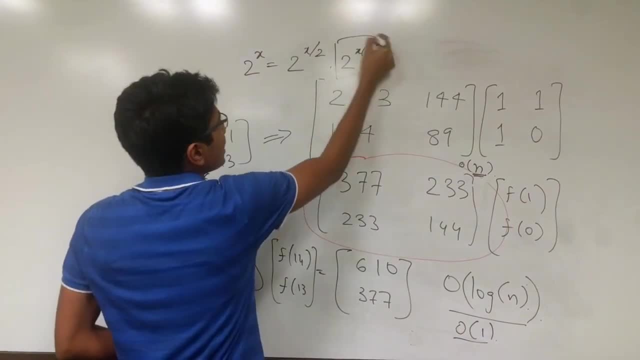 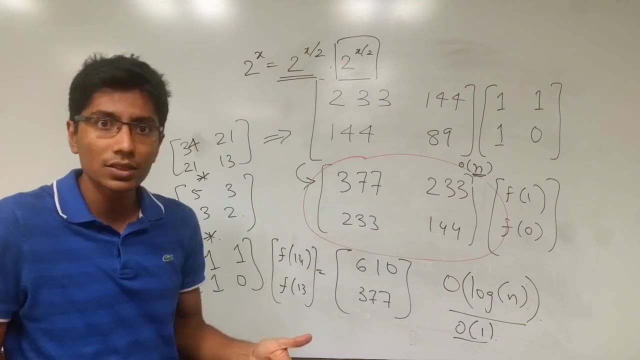 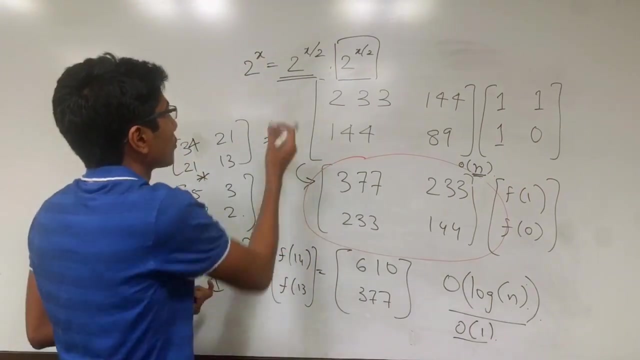 by 2.. Now we don't want to calculate this again if you have already calculated this part. That was the dynamic programming. It was recursive, it had no cycles. If you solve for this part optimally, then you're guaranteed that the overall solution is also optimal and of course there was optimal substructure.